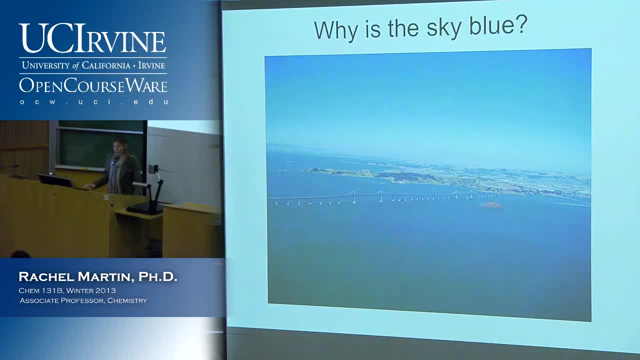 about the different ways that light can interact with matter. So before we do that, does anybody have any questions left over from last time, or about anything? Yes, Well. so the question is: if there are equations in the book and they're not in the lecture, do you need to know them? 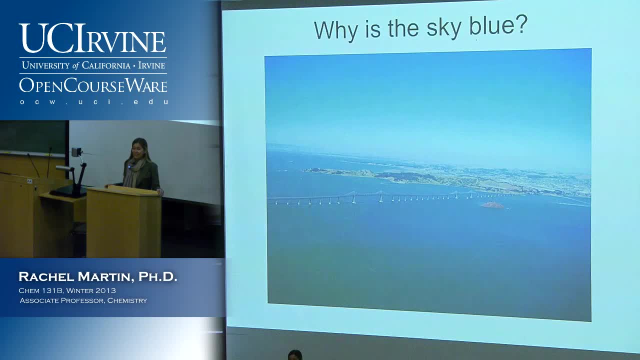 The answer is maybe. So things that are going to be covered on the test will be the stuff that we do in class, things that your TAs cover in discussion. those are also important concepts and things that you need to be able to do. 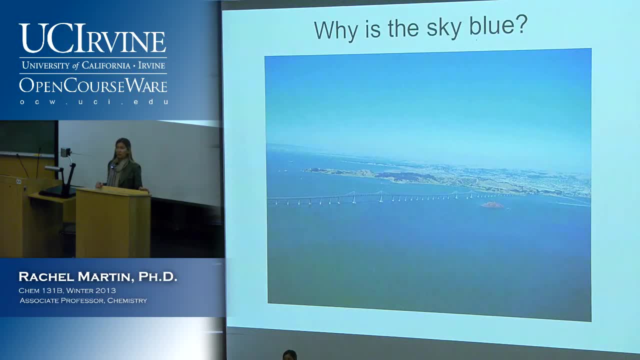 to do the practice problems. So a lot of times in lecture I'm going to focus on just trying to make sure that everybody understands concepts. That's what we're going to do today, And we might not necessarily get a chance to do examples of every particular kind of problem that you might need. 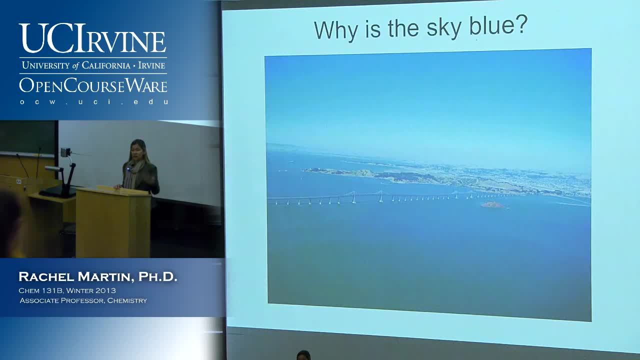 to do. Hopefully you get a chance to do that in discussion. The practice problems will give you an idea of what you need to do. There are other things that are in the book and you know that's just there for your information. 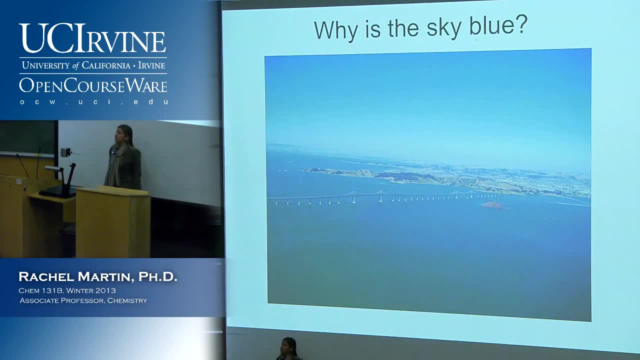 Does that help? OK. Anything else, All right. Let's start talking about how light interacts with matter. OK, So what I want to go over today is the difference between the two of them is: 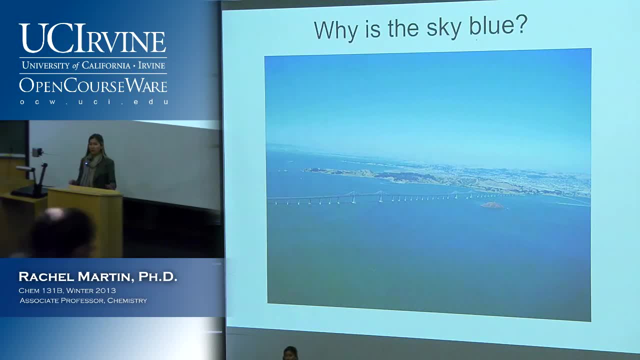 the difference between absorption and scattering, So this is something that people get confused about. It's one of the main concepts that we need to learn in P-Chem to understand the different kinds of spectroscopy that we use. And I want to put it more in terms 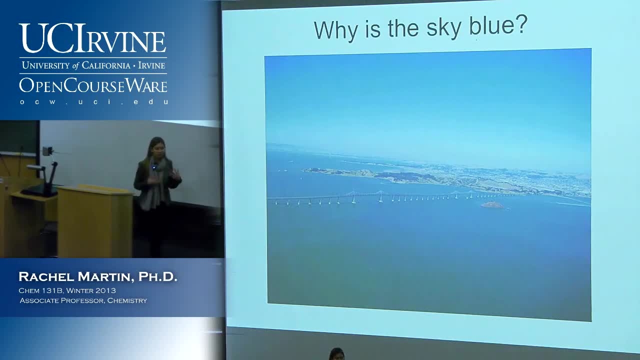 of things that we see every day. So you know again, it's all about photons interacting with matter And there are lots of different complicated formalisms to describe the things that can happen In specific cases. But what it boils down to conceptually is: 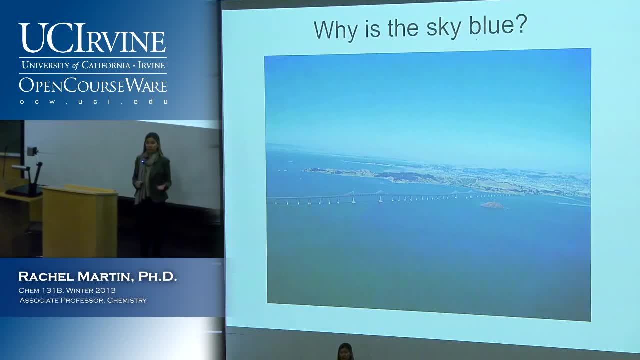 that if a photon interacts with matter, it can do one of two things: It can get absorbed or it can be scattered. So you know, it either gets absorbed and causes some kind of a transition in the atom or molecule, or it can bounce off. 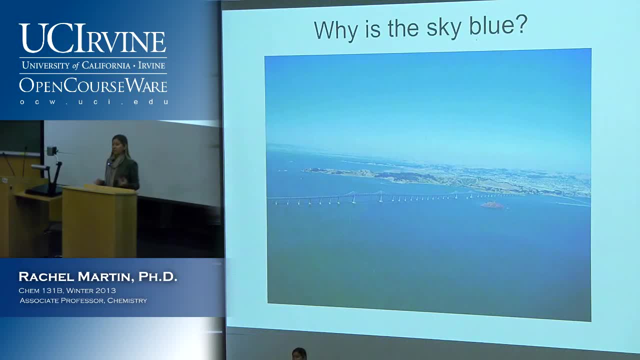 And it can scatter elastically or inelastically. We'll get into that toward the end of the lecture, But for right now I want to use some sort of familiar concepts to introduce just the idea of what's the difference between absorption and scattering. 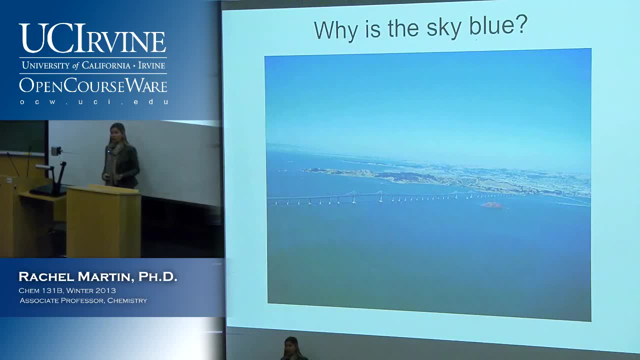 And there are some things that are obvious here and there are some things that are not obvious. So, all right, we're going to start with the basics. Why is the sky blue? Rayleigh scattering, Rayleigh scattering, That's right. 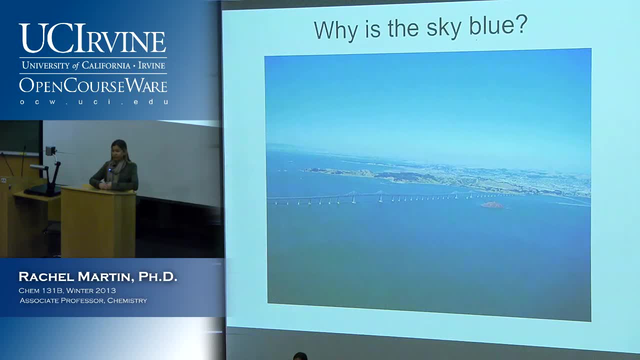 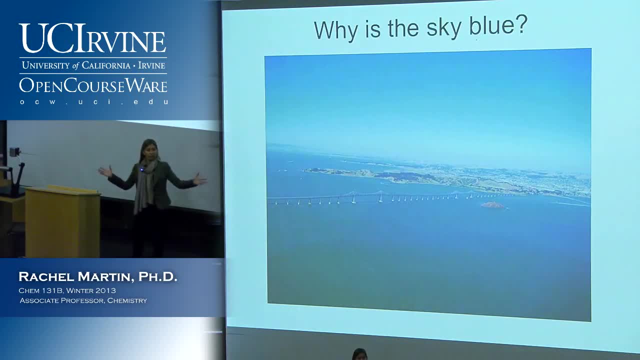 So if we have all the light just scattering off particles in all directions, why does it have a color? Does it wavelength scatter more than other things? Yeah, It has a really strong wavelength dependence. What are we scattering off, by the way, and really scattering? 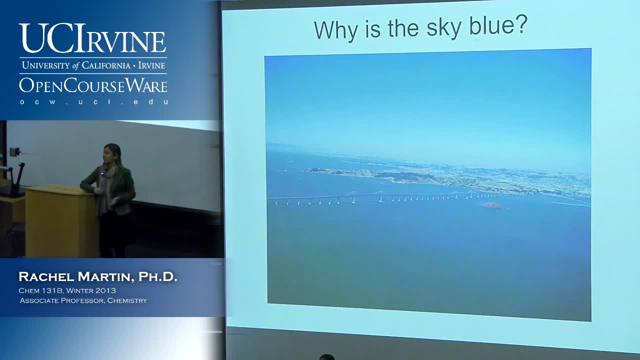 What's? what are the particles involved? Yeah, gas molecules, so mostly nitrogen, things like oxygen, whatever is in the atmosphere, All right. so what's happening here is the light is interacting with molecules or particles that are much smaller than the wavelength of light. 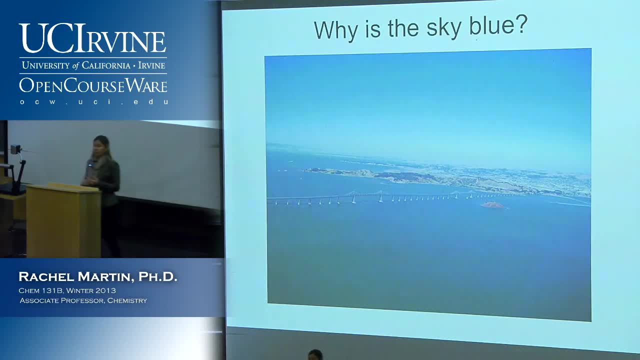 So remember, we know that, you know, we know the wavelength range of visible light is, you know, hundreds of nanometers. Molecules are a lot smaller than that, And so Rayleigh scattering is the solution to Maxwell's equations that describes what happens. 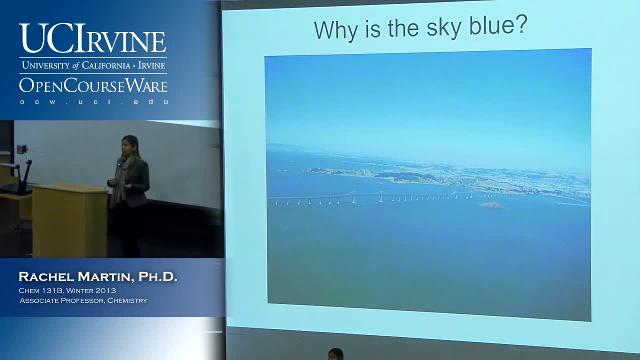 in that limit when the scatterers are much smaller than the wavelength of light, And so it has a really strong wavelength dependence, and what that means essentially is that smaller the small particles look a lot bigger to blue light than they do to red light. 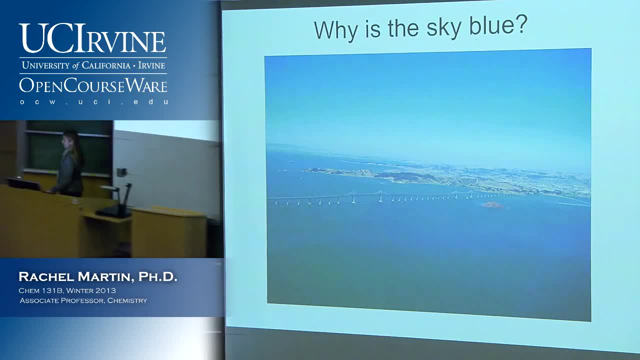 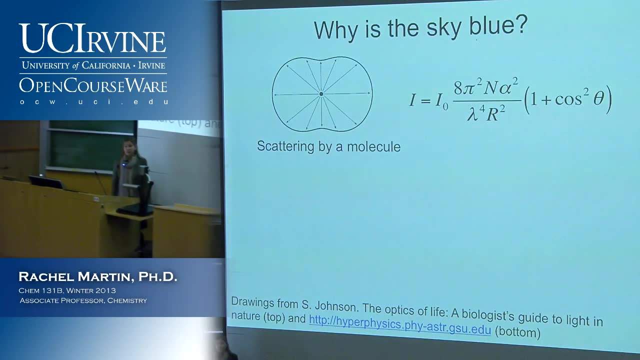 And so we get everything scattered and we see this nice blue color. So here's the functional form. just to remind you, if you haven't seen it recently: It has an inverse dependence on lambda to the fourth, So that's why we have this extremely strong wavelength. 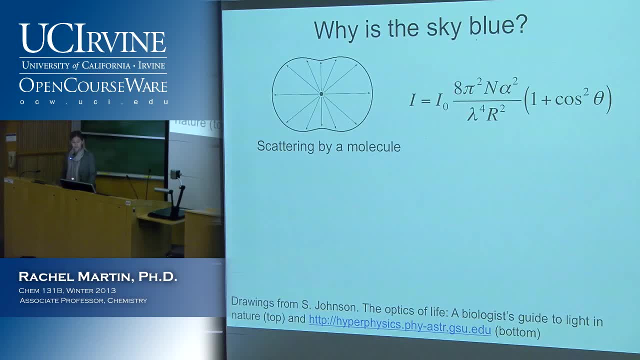 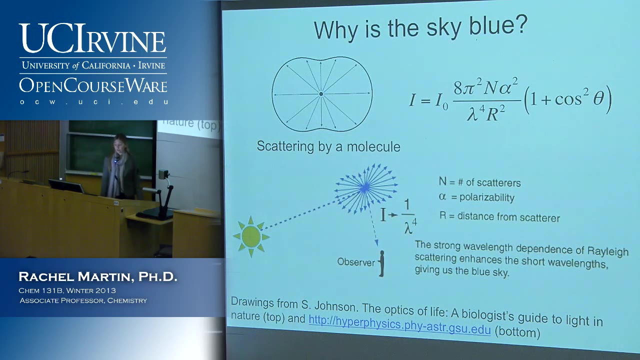 dependence, and it also has an orientational factor. So if we look at our little molecule, we see that there's more light scattered forward and backward than down, And so we can see that there's more light scattered forward than down, And so here's how we see this. the blue sky. 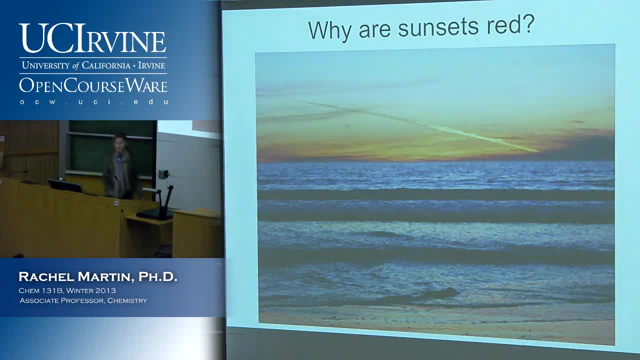 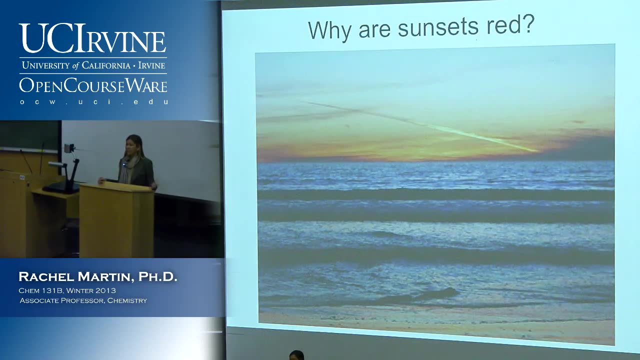 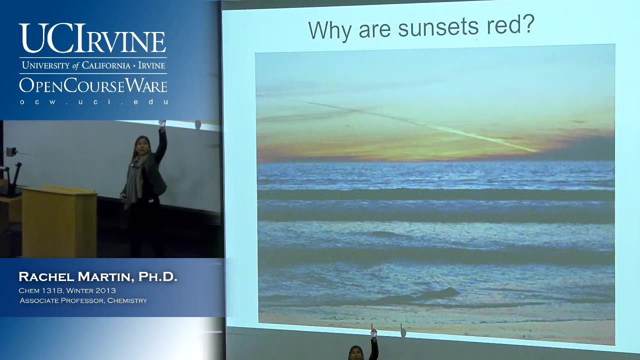 OK, So related issue: Why are sunsets red? Exactly So, we still have Rayleigh scattering, but now, you know, instead of having the sun overhead, it's on the horizon, And so it has to travel through more of the atmosphere to get to us. 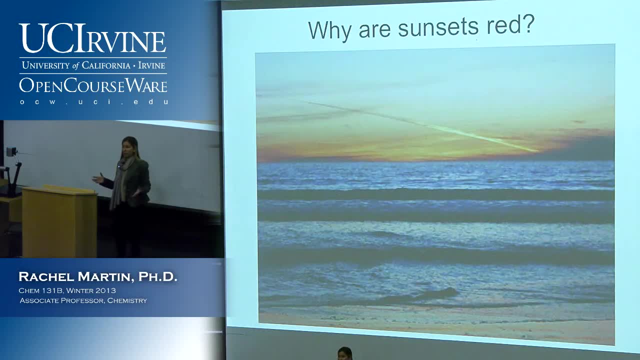 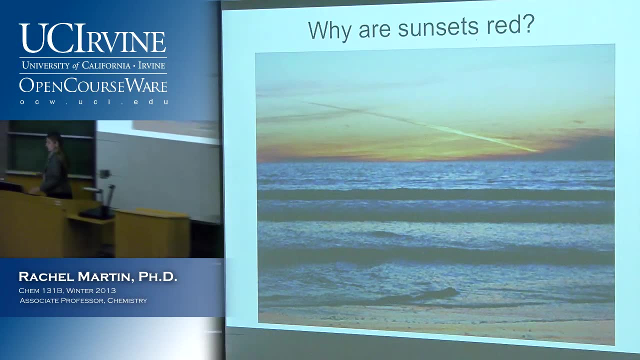 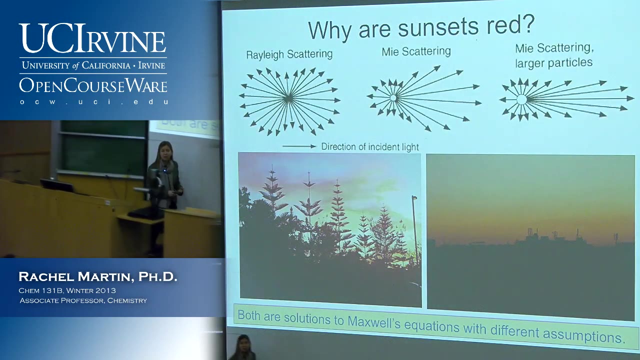 So we still have the same wavelength dependence, but all the blue light has already been scattered out and what we see left are the reds and oranges. So that's part of the story. There's also Mie scattering, which is what happens when you get particles that are larger. 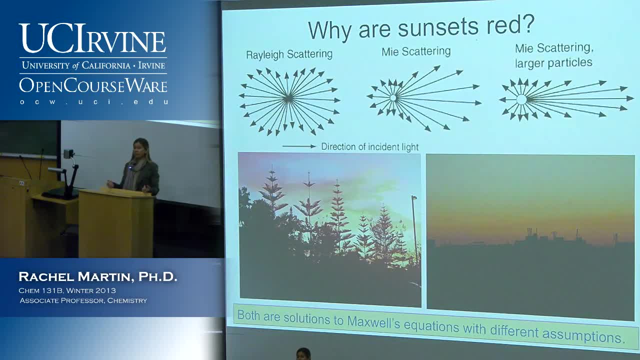 than the wavelength of the light, And in that case much more of the light is scattered forward and Mie scattering does not have a wavelength, It does not have a strong wavelength dependence. So this is really responsible for the for just scattering of white light in effects like when it's foggy. 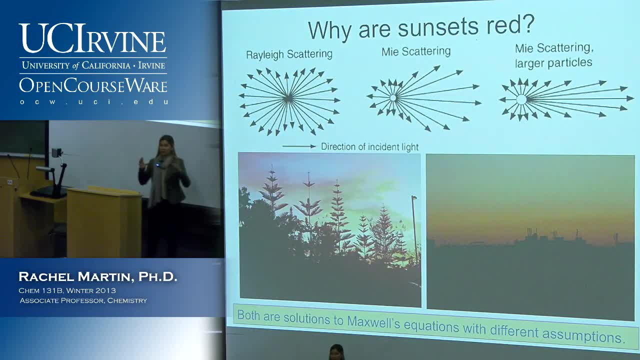 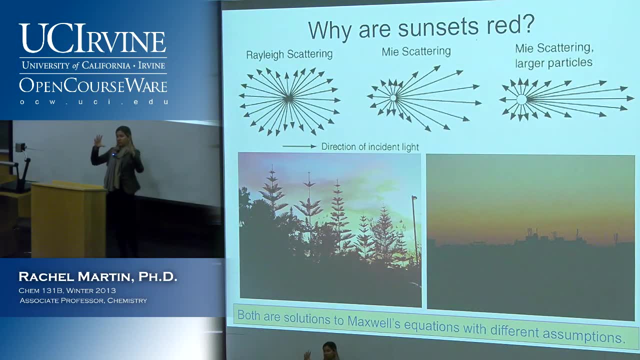 you see halos around street lights and things like that, That's because you know, in order to get to your eye, that photon is, you know, bouncing off these little particles, And so you see the, you perceive the street light as being. 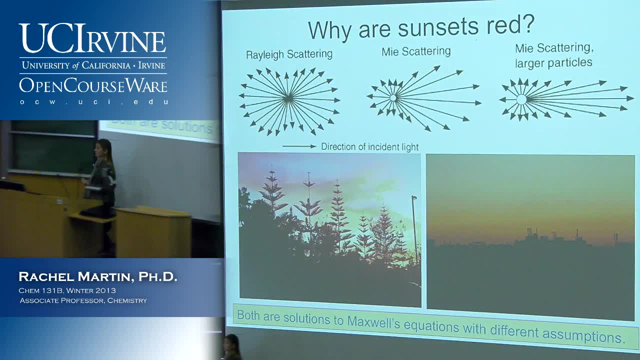 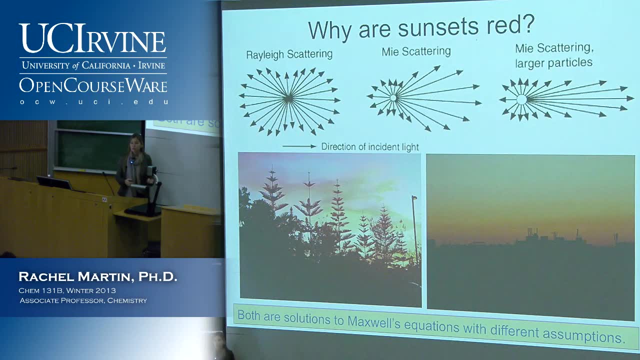 you know, larger than it actually is, because some of these photons are getting bounced off little water droplets that are in the air. So you often hear it said that pollution makes the sunsets more red and more beautiful because you have more scatterers. 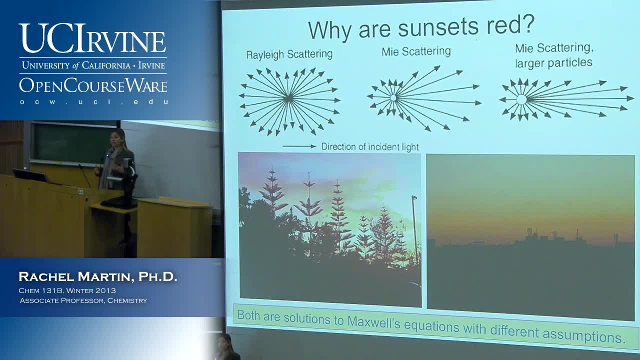 So is that true or not? The answer is it depends on how big the particles are. So if they're small, then they're contributing to the Rayleigh scattering and you see the more brilliant red color, whereas if they're larger, so if we have larger aerosols- 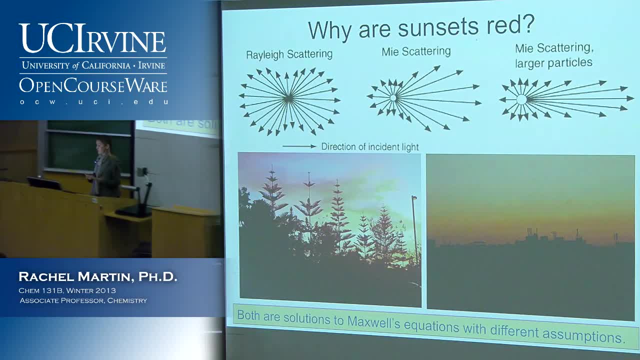 then that's just adding me scattering. so like this the picture on the right. it just makes everything kind of duller and in some cases it can make the colors softer. You can get more pink and tones like that rather than bright red. 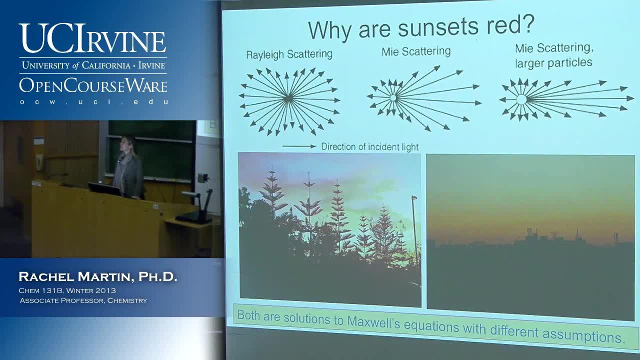 There was a question in the back. I was wondering: what do you mean by the scatters are of smaller wavelength than the light? Do you mean they absorb smaller wavelength? No, I mean the physical size of the particles is smaller than the dimension of the wavelength. 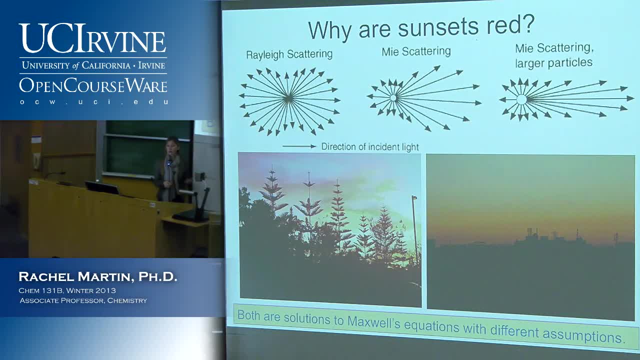 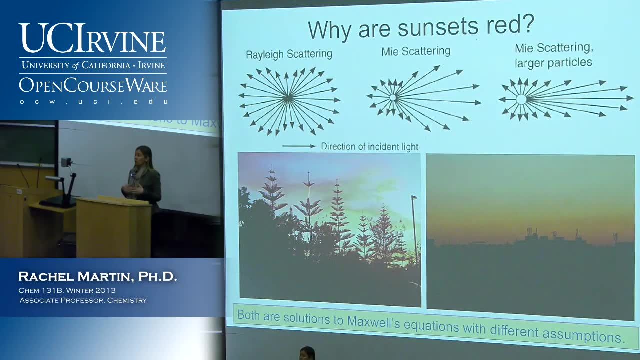 The wavelength of the light, that's all. So it matters whether we're talking about molecules, so those are obviously much smaller, These are Rayleigh scattering- or if we're talking about larger particles, so like gas, so sorry, vapor droplets. 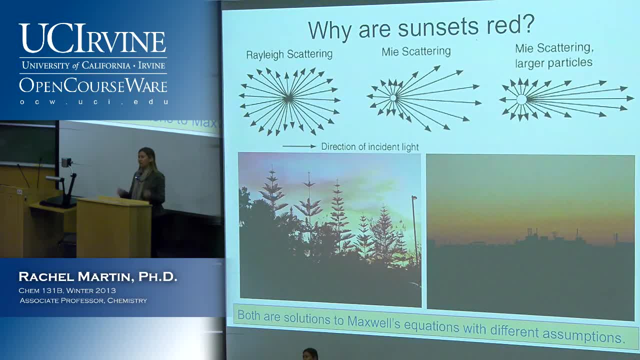 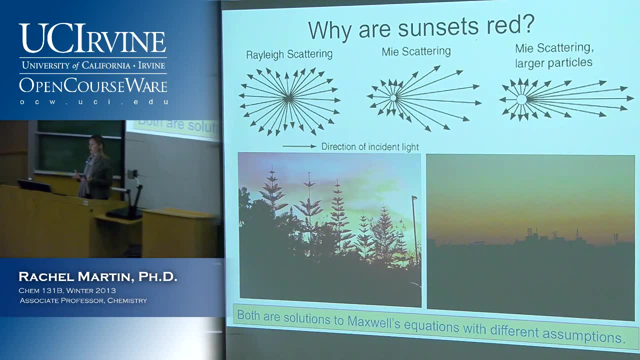 Yeah, liquid droplets that are suspended in gas like a cloud or fog. those are larger scatterers, and there are some pollution particles, aerosols- that fit into that category as well. OK, So it's also important to remember that both 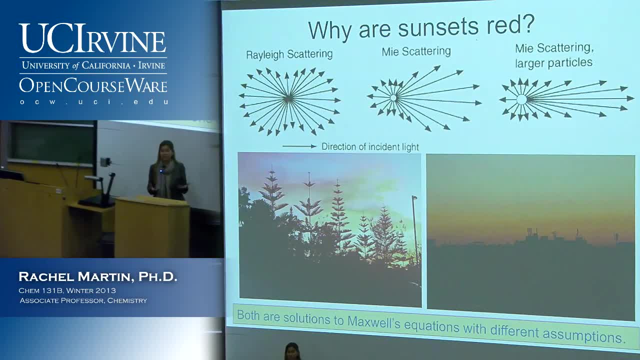 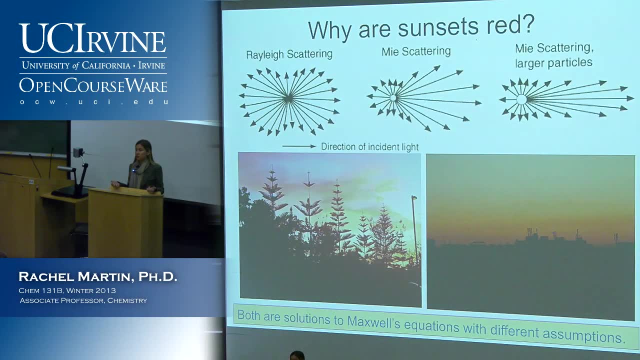 of these things are not different phenomena. It's the same thing. It's just there are different assumptions being made. They're in different regimes. We're just solving Maxwell's equations and we're making the distinction between: like: OK, if we're in the regime where the molecules are much smaller. 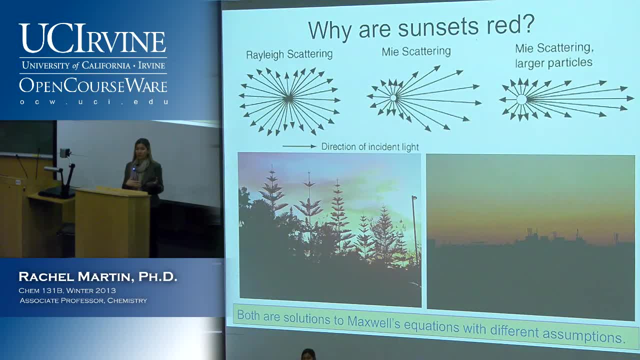 than the wavelength of the light, then we can make a certain set of assumptions, and if they're larger, then we can make another set of assumptions. If they're about the same size, then weird things happen. It's pretty interesting, But remember that these people didn't have computers. 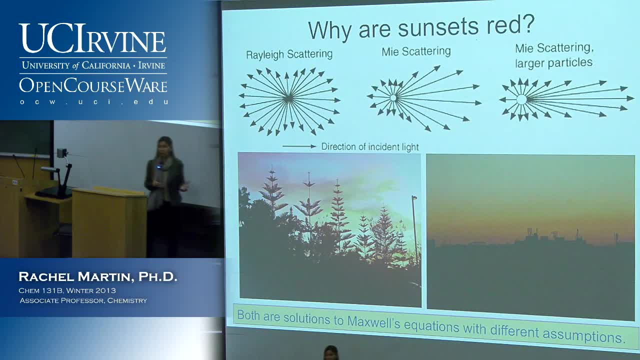 when these things were discovered. So it was really. you know, getting any sort of mathematical form to anything was a really hard one, And so that's why we have all of these things that are treated as though they're different phenomena, when you know. 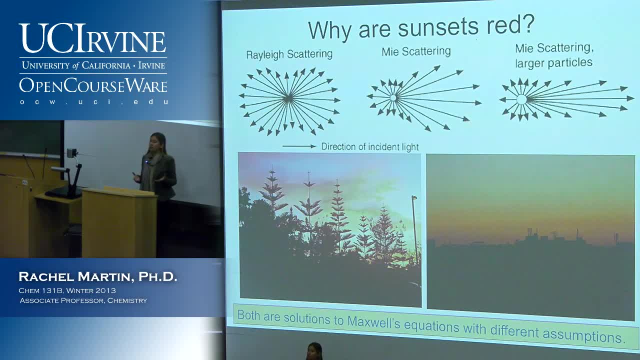 actually, at this point we can just stick it into Mathematica and solve it. So it does a lot of times. this is taught, you know, as the same way that we do it. It's the same way that it came out historically. 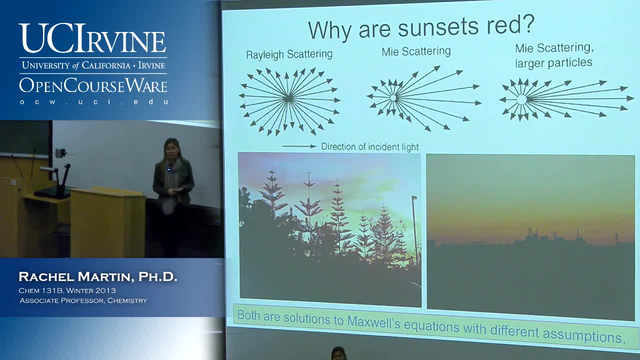 where we have these different regimes and that's fine. Those are convenient approximations that you can use. But do remember that it's all the same phenomena And I'm not giving you a nice, pretty functional form for me- scattering, and that's because there really isn't one. 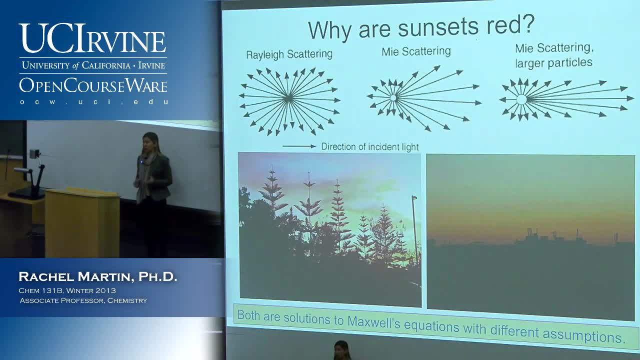 If you want to do that, there are programs that you can use to do it, but computational methods are the way to go there. Yes, Sorry, this is off topic, but how does the northern lights work? How does the northern lights work? So that's there are you know. 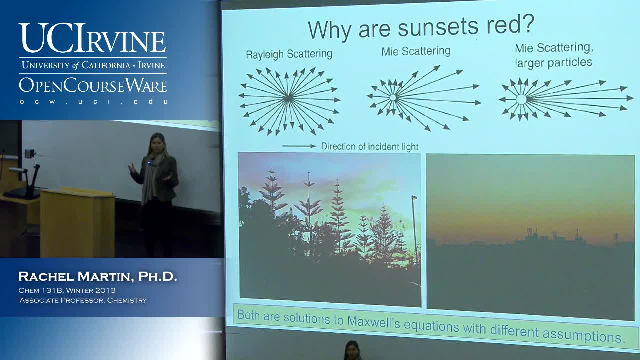 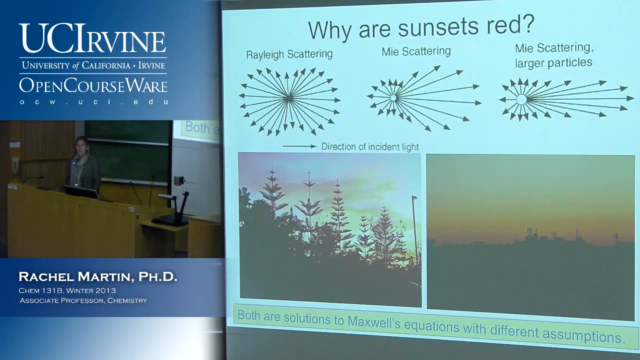 there's a number of different ways to do it. There are ionized particles that are emitting radiation, And you know what. we'll talk about that when we get into electronic spectroscopy. We'll save it for later. OK, So we have covered the somewhat obvious. 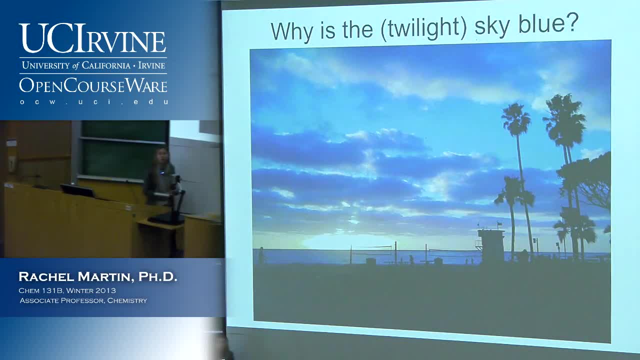 Let's get into less obvious. Why is the sky blue at twilight? So remember we have our nice Rayleigh scattering explanation for why the sky is blue overhead. So our sun is up here, The light is scattering down to us. We see the blue light. 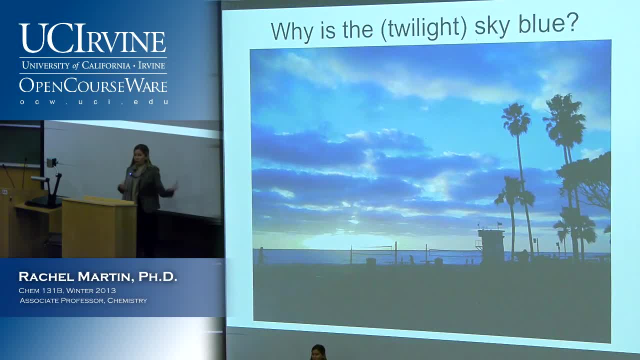 Then it's on the horizon. It goes through a longer path length, There are more particles in the way and now it's red, But the sky is still blue, even though the sun is not up there anymore. What's that about? So the answer is: a lot of it is due to the color of ozone. 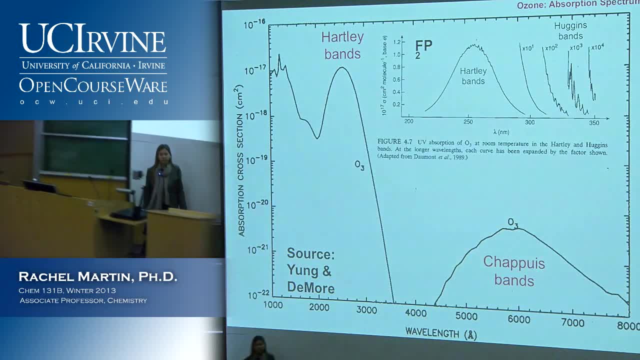 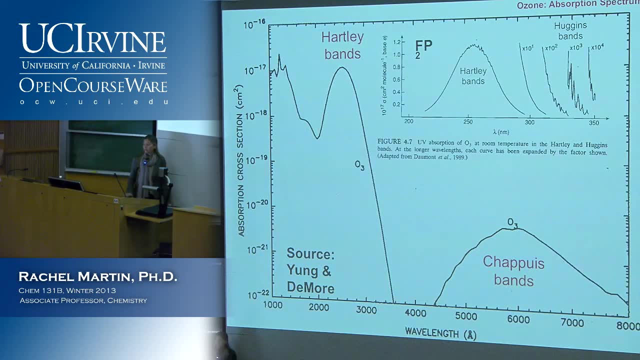 So here's the absorption spectrum of ozone And you can see this. you know, again, these things have historical names. The Hartley bands are in the UV and those are really big. But then there's this little smaller band, the Chapuis bands, that are kind of more in the visible region. 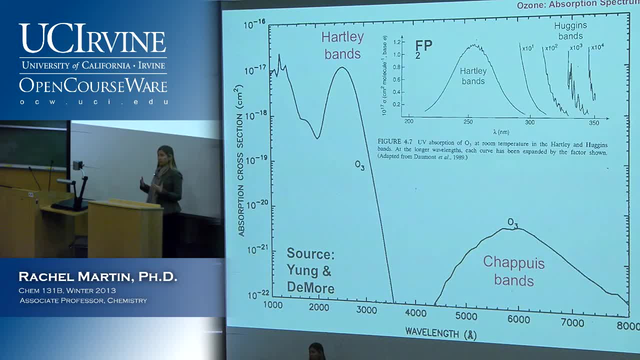 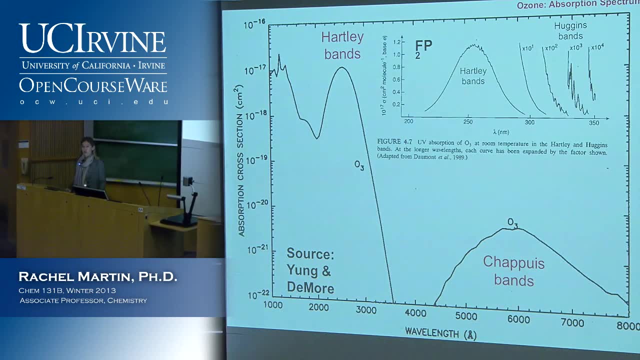 So ozone is actually absorbing and it has a color and it's blue. So you know again, remember, when we say something absorbs and has a color, it's absorbing everything but blue. So that's what we see. That's something that we're going to talk about again. 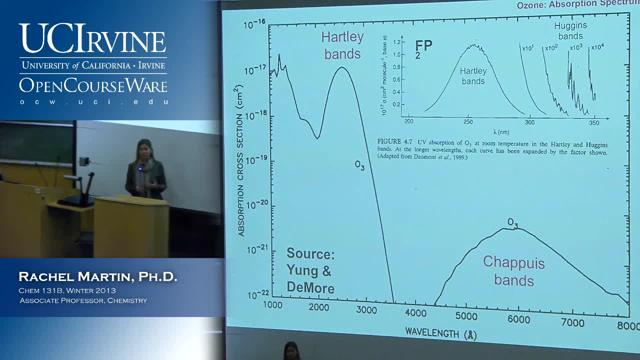 when we get into electronic spectroscopy, The details of how we perceive color and how we talk about it are natural to our perceptual system. But when we go to think about spectroscopy and what we can measure with instruments, it's not necessarily the best way to describe things. 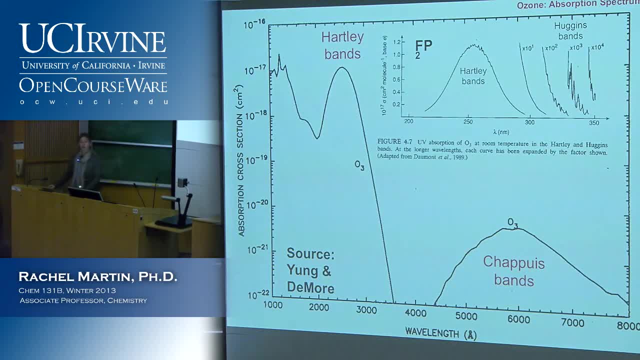 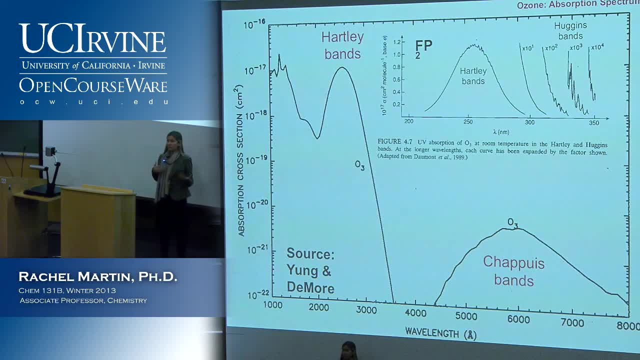 The blue is blue, But we get similar effects. What we perceive can be the same, whether it's based on scattering or absorption. The sky looks blue to us either way And you know, a lot of us have never thought about why it's blue. 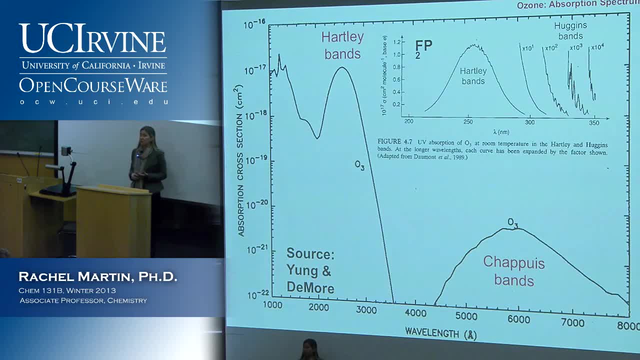 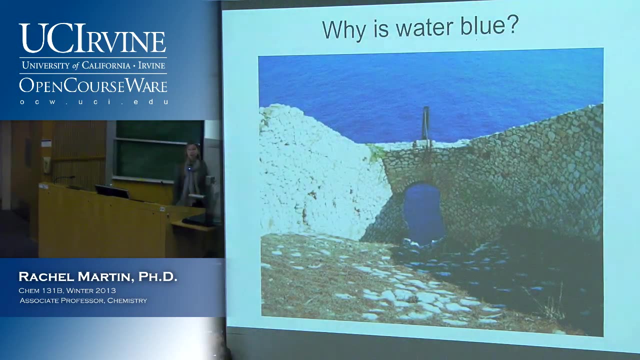 at twilight, when you know the mechanism looks like it might be different, But these are different phenomena And, again, these are the only. these are basically the only things that photons are going to do when they interact with matter. OK, So why is water blue? 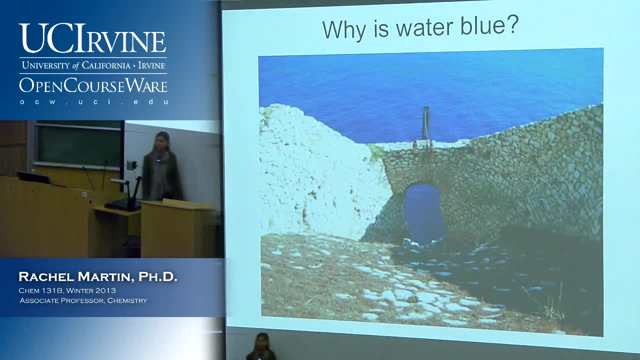 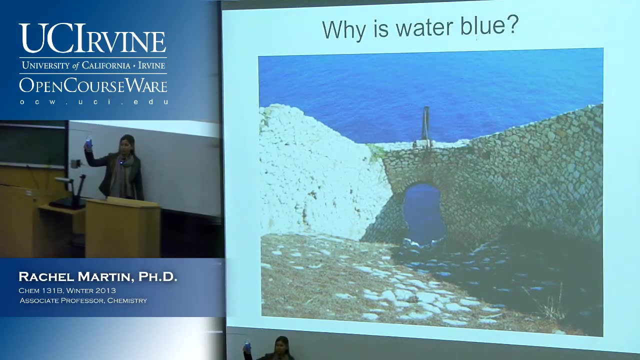 And particularly if I have my bottle of water, it looks transparent, you know, except for where it's going through the, where the light's going through the blue label. But if we look at the ocean or a large amount of water, it looks blue. 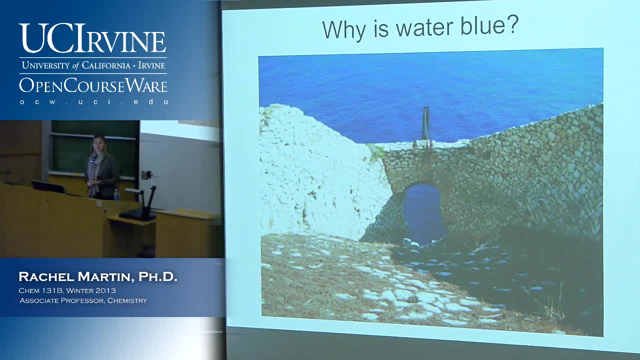 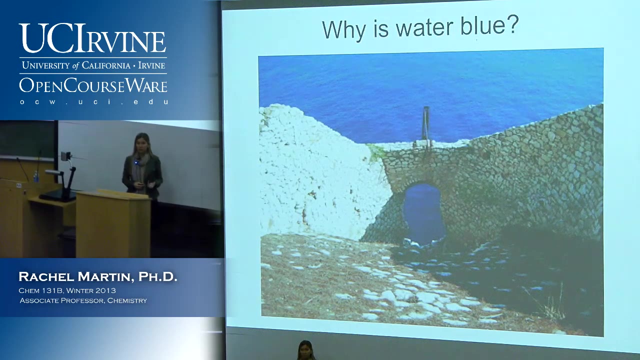 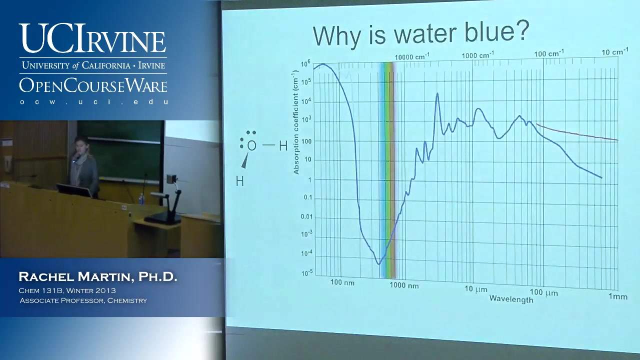 Why is that So really scattering? again, that's, it's part of the answer. So it turns out that water itself is actually blue, very weakly. it's weakly absorbing, And I will show you its spectrum. So here is just the, you know, the overall absorption spectrum. 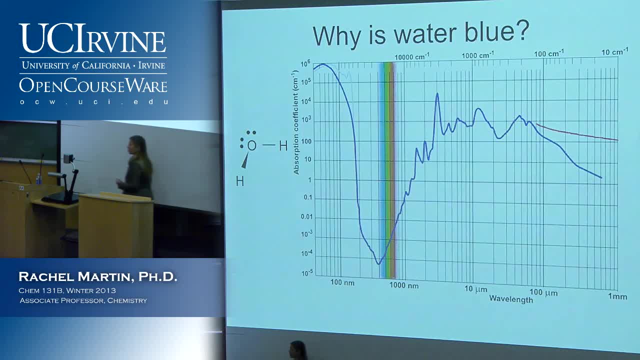 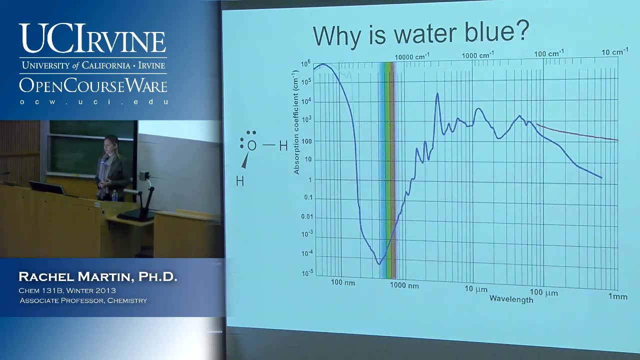 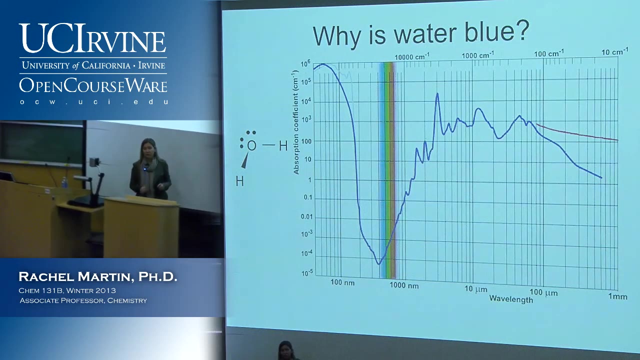 of water, with the visible region drawn in there And you know notice it has, you know, notice it has giant absorption bands at both longer and shorter wavelengths. There's just this really narrow region where it doesn't absorb very much And if you look at where the water starts, does start. 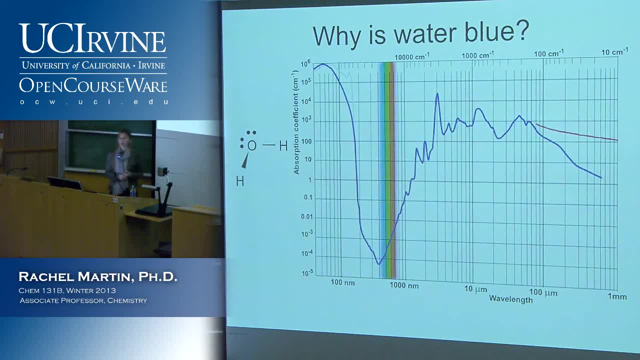 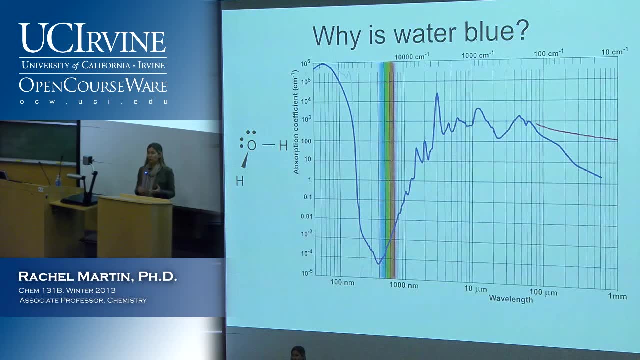 to absorb. in the visible region it's absorbing out most of the red, So it is very weakly blue, And the reason that it looks transparent when you have a small amount of it is that you just don't have very much, Whereas when you get it in a more bulk quantity. 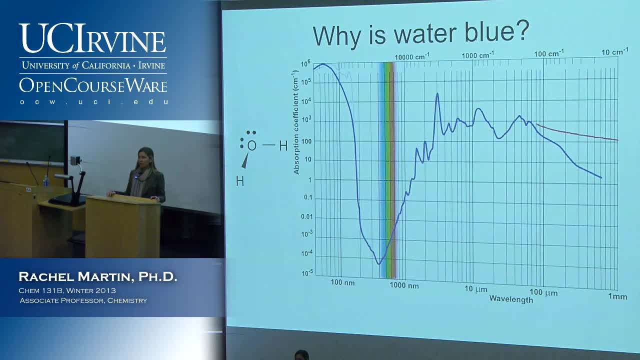 you can actually start to see the color. Now we need to get back to the issue of scattering, Because if that was the whole story, if we just had the weak chromophore, then water wouldn't look blue when we look down on it, right? 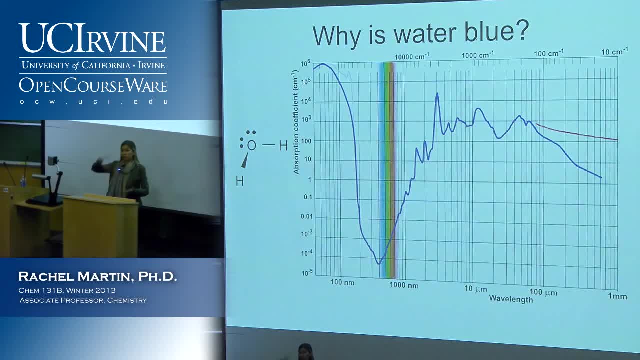 If we went scuba diving and looked up, we would see blue water. But if it was just absorbing when we look down on it, it would always look blue. It would always look black. When we look down and see the blue water, a photon has to go. 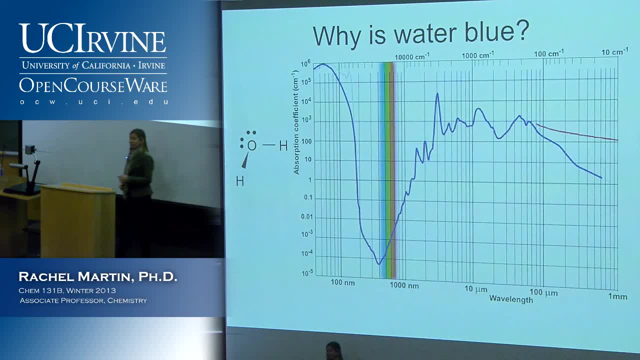 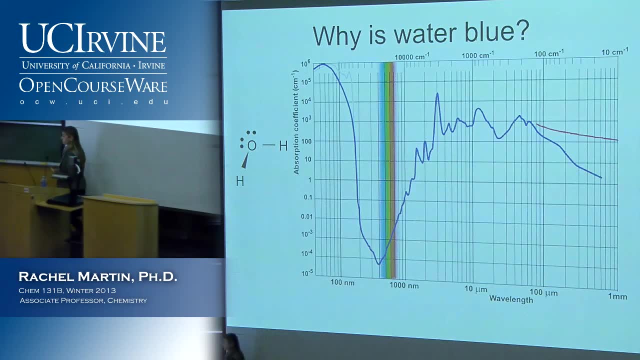 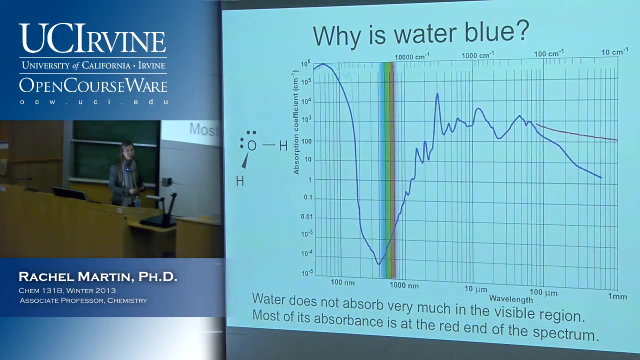 in there, bounce around and then come back out to our eyes. So scattering definitely does have to be part of the answer. So the answer there is both. Another thing that's pretty interesting to think about is a couple of issues involving the 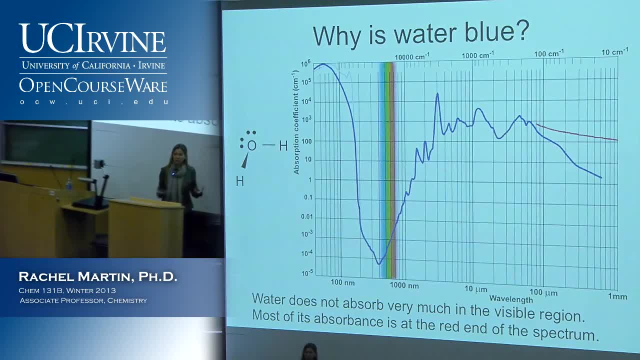 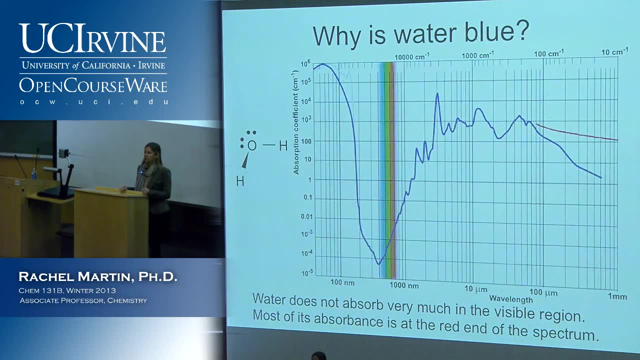 this spectrum. So one is, if you look at this absorption spectrum of water, you know we've got strong absorptions. you know both above and below the visible region It's. you know, it's kind of an interesting coincidence. 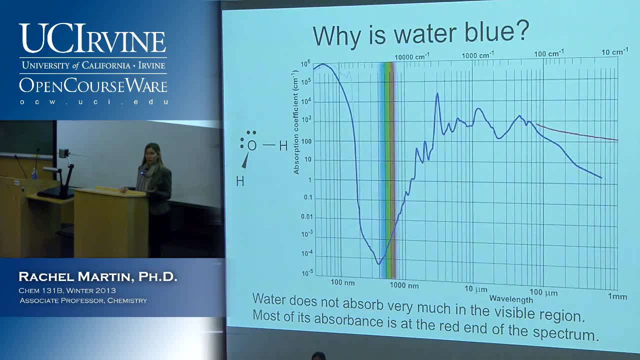 that there is any region where water is transparent, and you know so, visual systems in humans and all kinds of other animals were able to evolve. If the spectrum of water didn't look like that, we wouldn't be able to see, because you know. 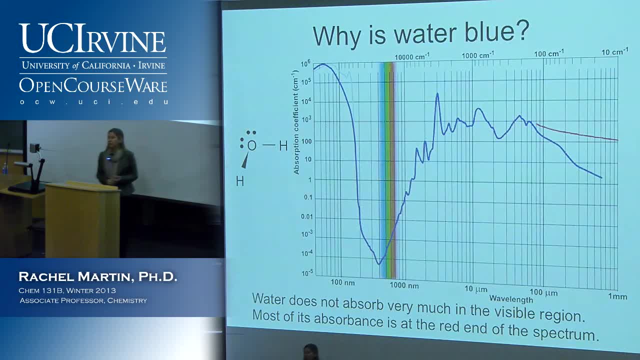 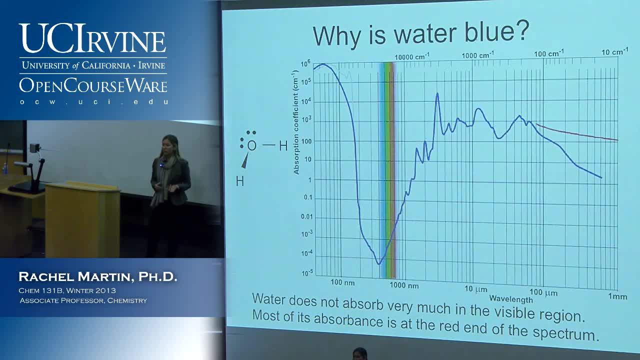 Another thing that I'm not going to get into right now, but I want to point it out, is: why is water transparent? It, you know, or glass or other media like that. it's not that the photons are just bombing through without interacting with anything. 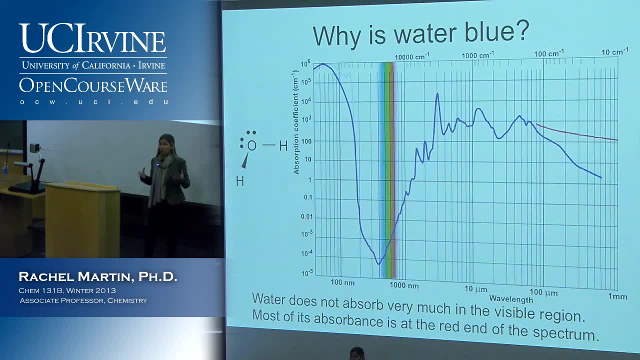 And if that doesn't confuse you, it maybe should. So this is something to think about. If you want to know the more detail, detailed version of the answer, there's a little book by Richard Feynman called QED- Quantum Electrodynamics. 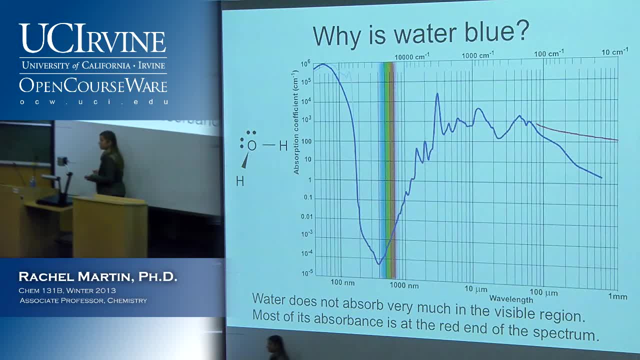 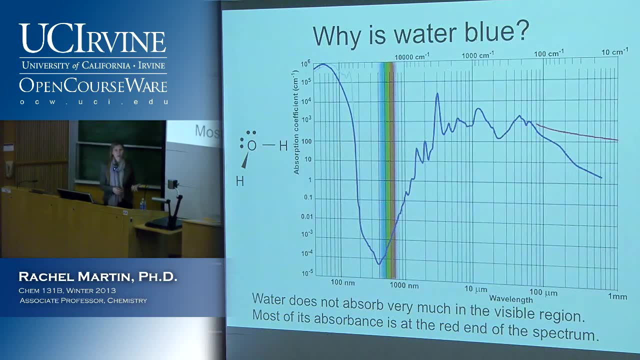 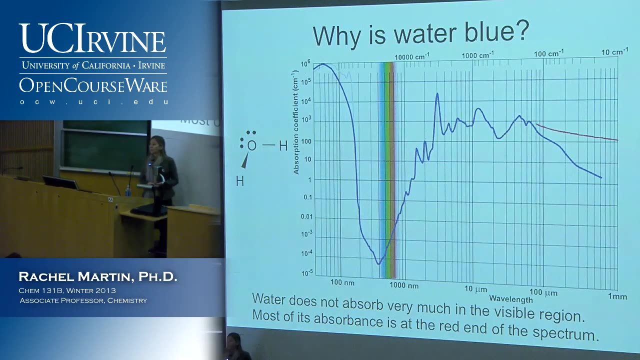 that explains all of this in a pretty intuitive way. That's a good thing to read, OK. So we've seen how combinations of absorption and scattering can produce these color effects that are pretty familiar to us. I want to talk about one more phenomenon that sort. 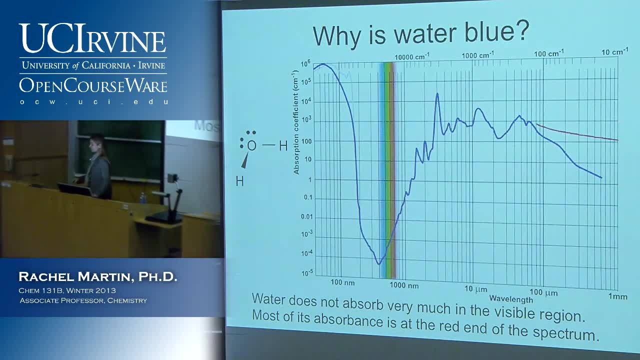 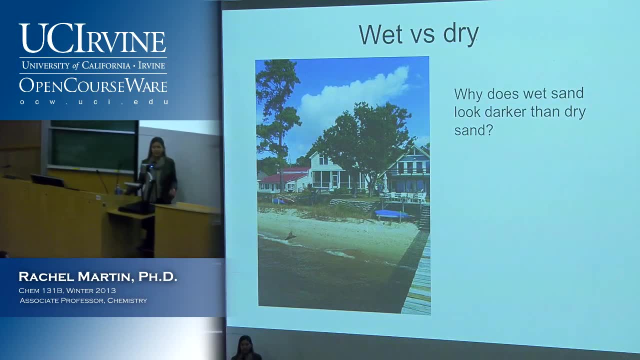 of illustrates the difference. which is why is it that when you put water on media, it looks darker? So, as we talked about, the water is transparent. It has a really weak blue color, but we don't see that in the thin layer. that would be on some object. 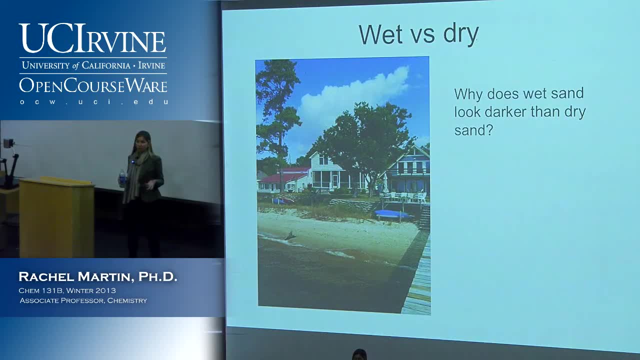 And when it evaporates, it, you know, doesn't leave that thin layer, It doesn't leave a stain, the pigmentation or whatever we're getting goes away. Let's think about why that is So. demonstration: Can everybody see that? 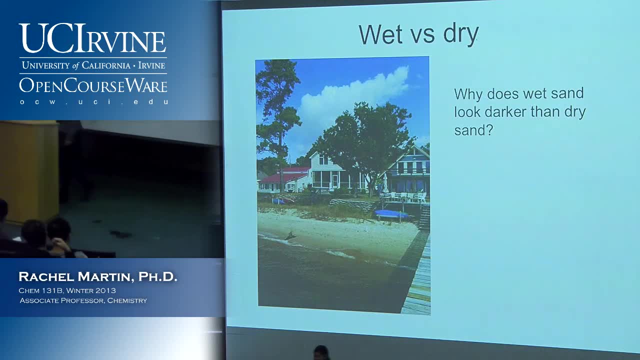 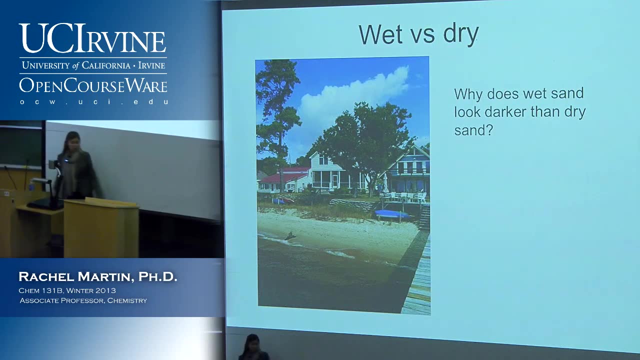 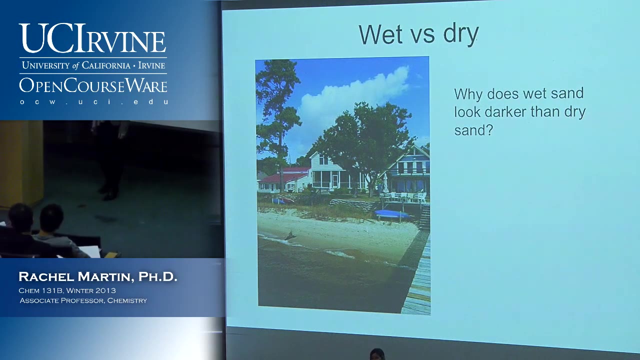 So it's just water. It's not going to hurt anything. As we discussed, it's going to dry and go away, OK, So why does it look like that? Why is it darker When it's wet and it gets light again when it's dry? 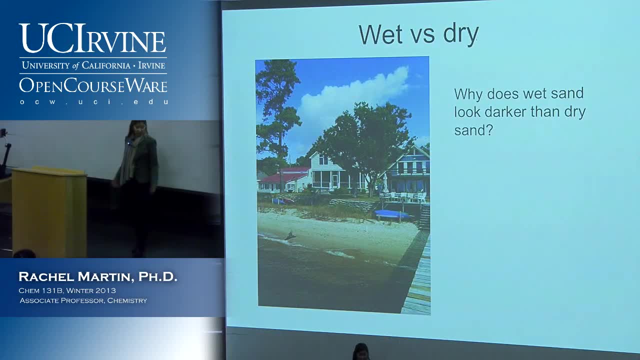 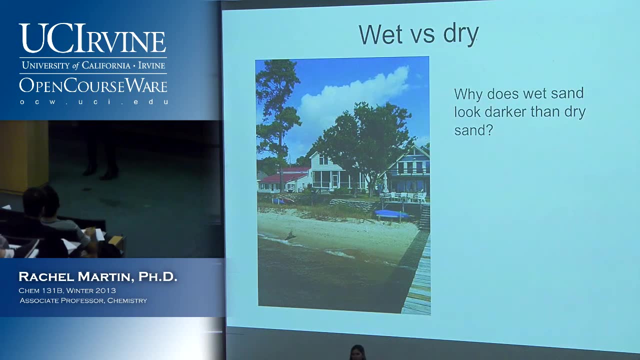 It's absorbing more. that's definitely true, but let's talk about why. OK, So let's go back to sort of the you know more physics interpretation of light. You know we've been thinking about photons. Let's think about light rays for a minute. 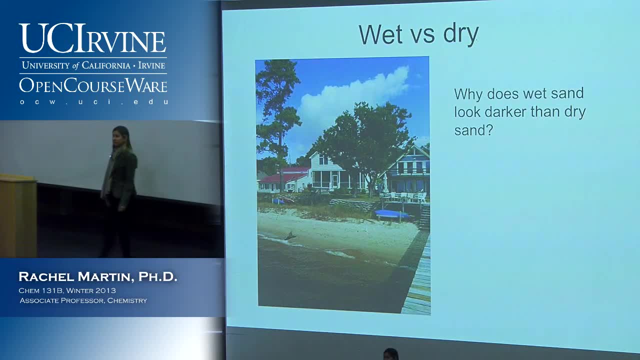 It's another, perfectly valid interpretation that explains some of these phenomena. So if we look at this, what's going on? there is the difference in refractive index between the air and the carpet is large, And so when light is coming, you know. 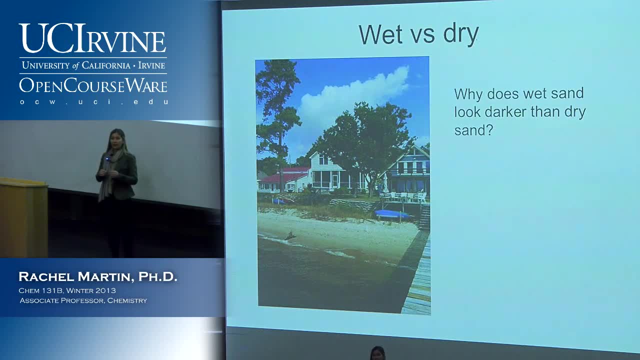 when light rays are coming from the air and they're going to the carpet, they get scattered a lot. These light rays get bent over a wide range of angles because there's more bending when you have a larger change in refractive index, When we saturate it with water. 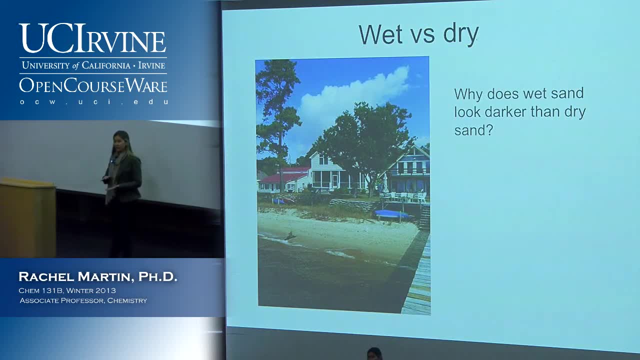 now the difference in refractive index between the water and the carpet is lower, So the light rays get bent a smaller amount, and so they bounce around more before they make it back out to our eyes. So basically, what's happening is, instead of just scattering right off, some of the photons are going. 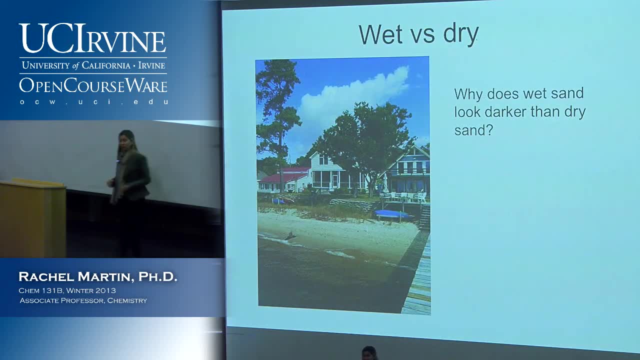 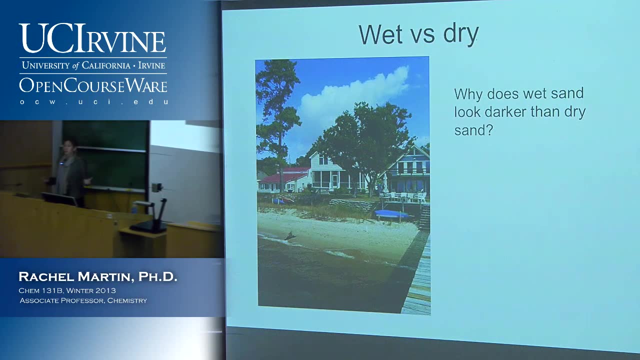 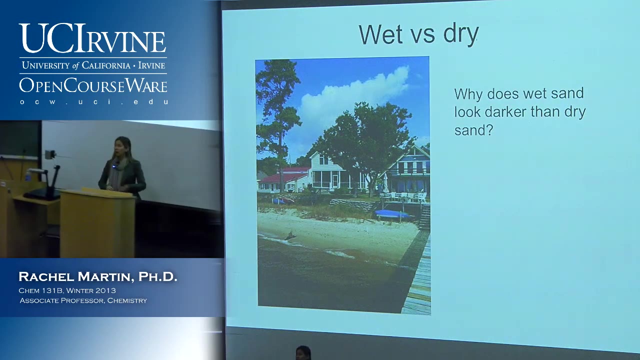 into the nether parts of the carpet, never to reemerge, and that's why it looks dark when it's wet. OK, So that is the difference between absorption and scattering. and now let's apply that to actual spectroscopy Question. Sorry, could you say that last part one more time? 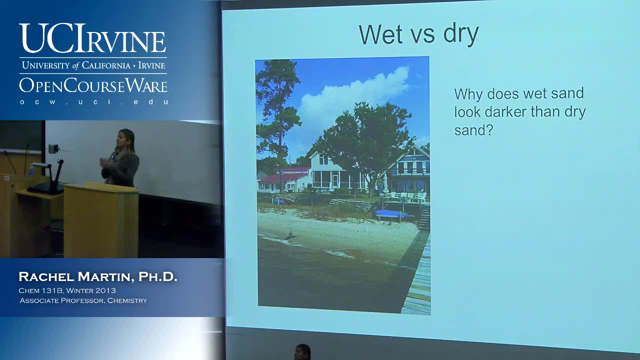 Sure. So when you Scattered more, Well, so it gets scattered at a wider range of angles. when it's dry, because the difference in refractive index is greater between the air and the carpet, Then when we pour water on it, that has a higher refractive index. 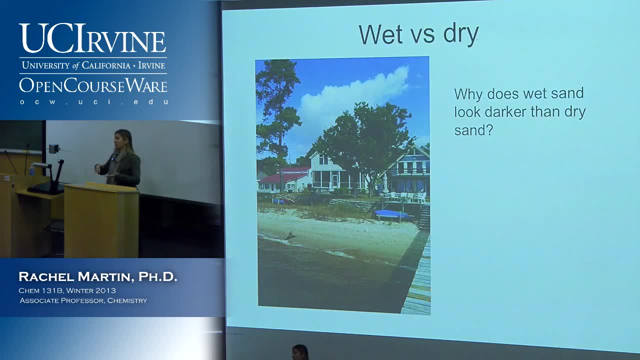 and so the difference is lower. The refractive index is less. If I poured benzene on it it would be even less, but that would be dangerous and I'd probably get in trouble, since it's on video. So you know we're making the refractive index difference. 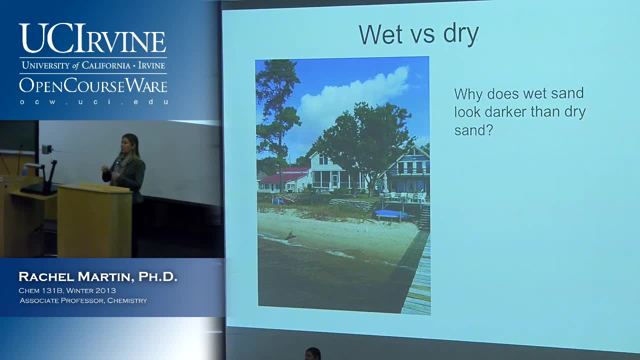 smaller between the- you know, the carpet and the surrounding medium, and so that means that the light gets bent under smaller angles and so it has to bounce around more and more before it gets back out to our eyes, and some of it gets absorbed before that happens. 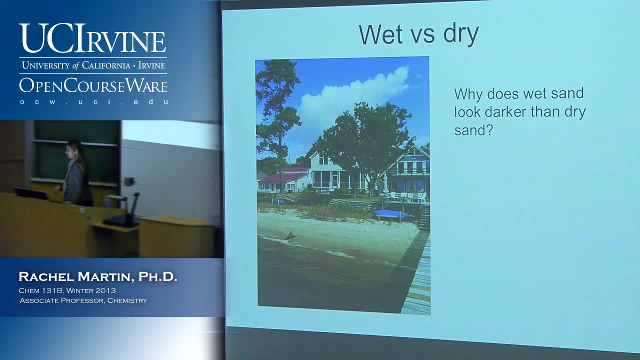 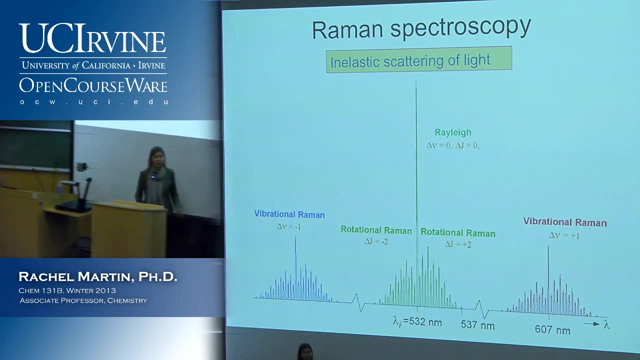 So that's why it looks like that. OK, So that's fun. but the real reason why I want to make sure everybody understands the differences between absorption and scattering and how they can give us some of the same phenomena, is that we need to talk about the difference. 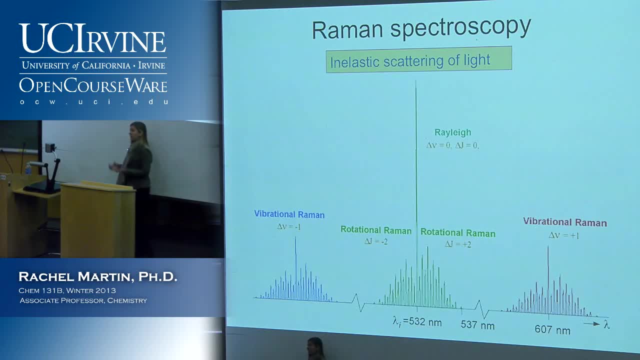 between absorption, types of spectroscopy and Raman spectroscopy. So Raman spectroscopy is what we get when there's an inelastic scattering of light. So when we shine light at something, if it doesn't get absorbed it has to scatter. we know that. 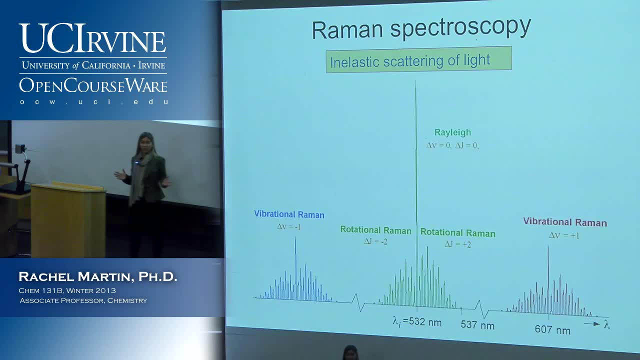 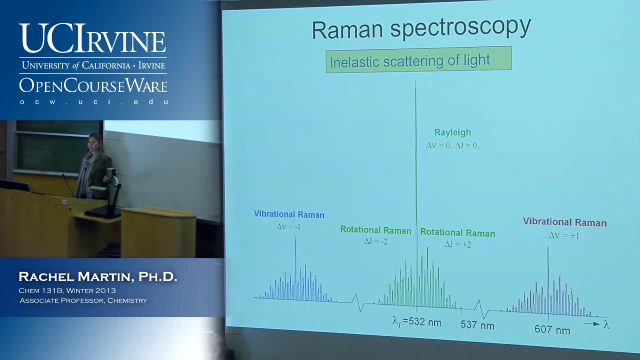 We already know that most of it just bounces right off. it scatters elastically. that's really scattering, which we understand. But what can happen sometimes is it can either the light could lose a quantum of energy to the molecule or it could take a. 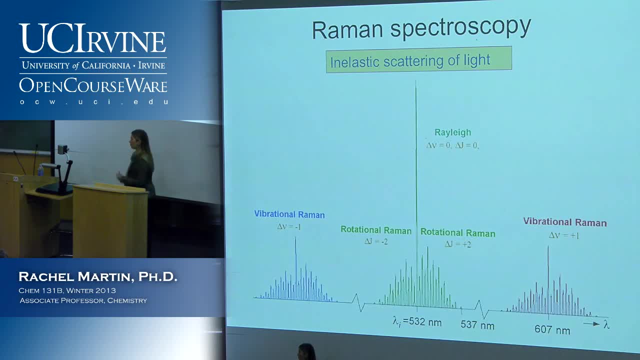 quantum of energy from the molecule, and when that happens we get a Raman spectroscopy, And so I'm going to put up this picture quite a few times as we go through our discussion of different types of spectroscopy. So we've talked about direct rotational spectrum. 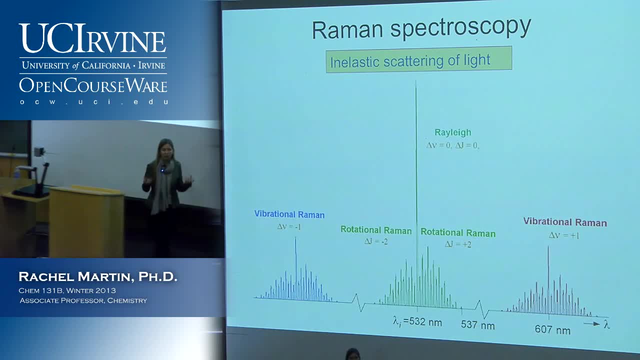 We've said like: OK, we need to have a dipole moment to see a pure microwave spectrum from the rotation of a molecule, because we're, you know, we're watching some part of the molecule go around and we have to be able to tell the difference with our electric field. 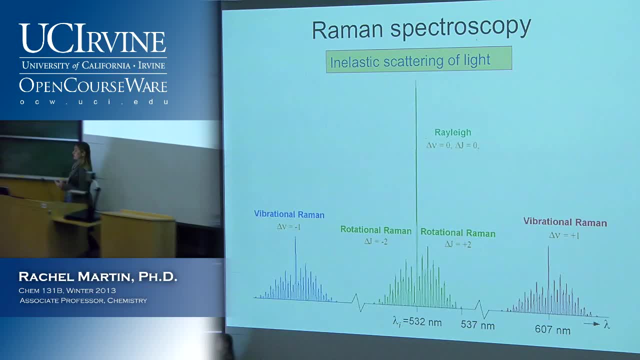 OK, So we're going to put up this picture quite a few times as we go through our discussion of different types of spectroscopy. Raman spectroscopy is a different effect. So instead of absorbing that photon and bumping the molecule up to an excited rotational state, 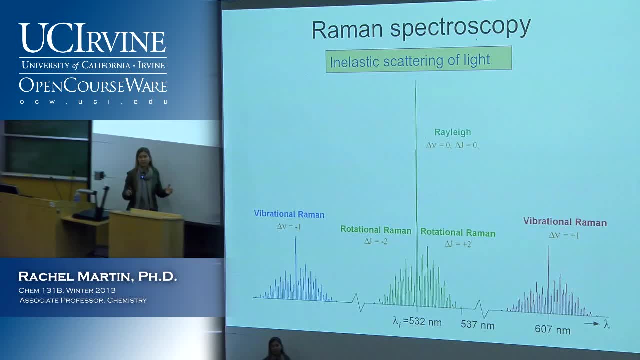 we're having the photon bounce off, but it doesn't scatter elastically. It either leaves behind a quantum of energy or it takes a quantum of energy from that molecule and in that way bumps it up and down in the rotational state. So this is rotational Raman. 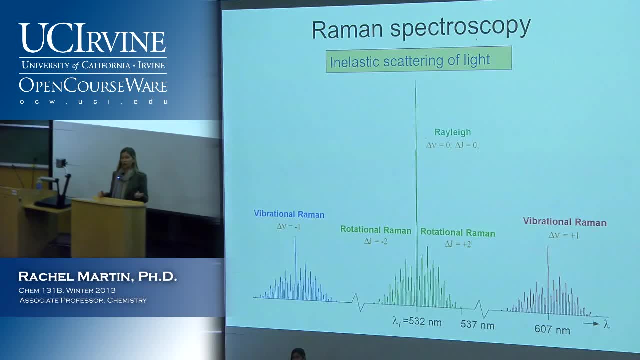 We can also have vibrational Raman, which we'll get to later on, And I just want to give some examples. This is sort of the big picture version of this. We're going to have, you know, rotational spectroscopy and vibrational spectroscopy, and there are two types of each. 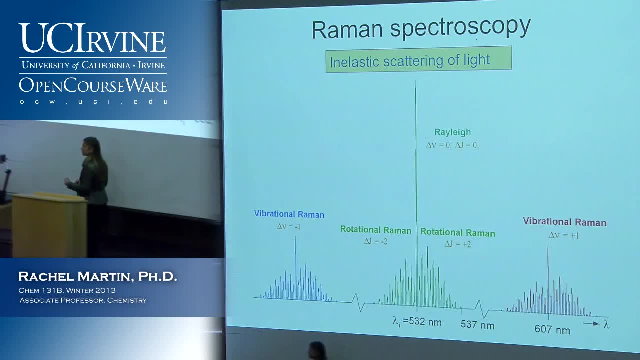 We can either have direct absorption or we can have the Raman spectra, which is based on scattering, And they have different selection rules and they give you complementary information. They're not identical. OK, So some terminology, The Rayleigh line- this picture is actually not drawn to scale. 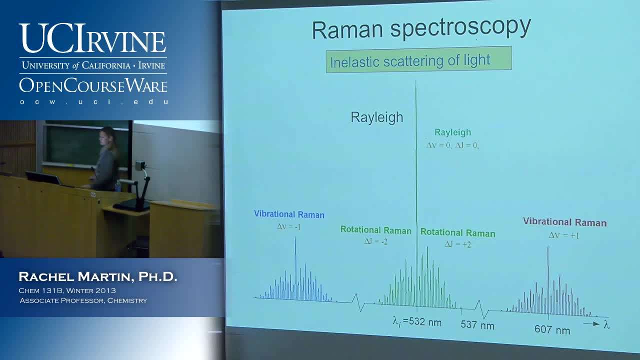 The Rayleigh line is way, way, way bigger. The Rayleigh line is much bigger than any of these Raman spectra And it also makes sense that when we're talking about vibrational Raman, those are off to the sides quite a bit. 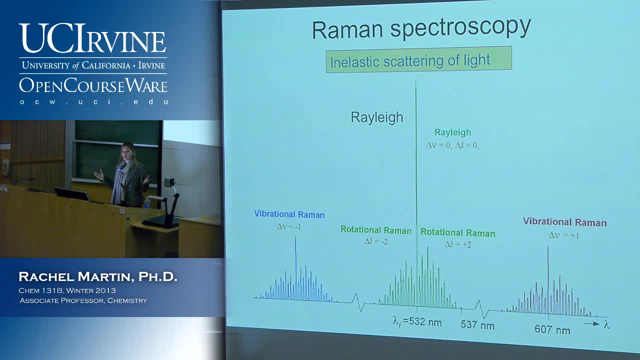 more and you see these breaks in the horizontal axis. It takes a lot more energy to excite vibrational states and it does rotational states. So for now we're just going to be talking about the rotational Raman spectroscopy, But this other, this picture is going to come back again. 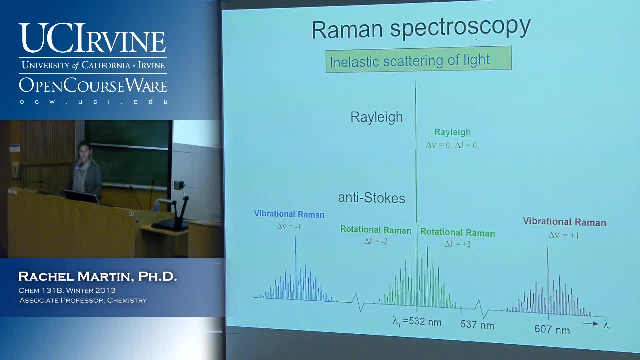 when we talk about vibrational states, So some terminology. We have the Stokes line and the anti-Stokes line, depending on whether the photon is losing energy to the molecule or gaining energy from the molecule. And you have to be careful because you will see these spectra plotted in terms 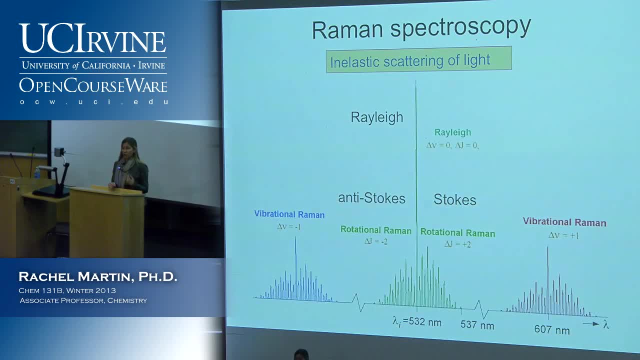 of wavelength, like this one is, And so remember that a longer wavelength equals lower energy. You will also see it plotted sometimes in terms of frequency, So a higher frequency, A higher frequency is a higher energy, And so which one is, which depends on how it's plotted. 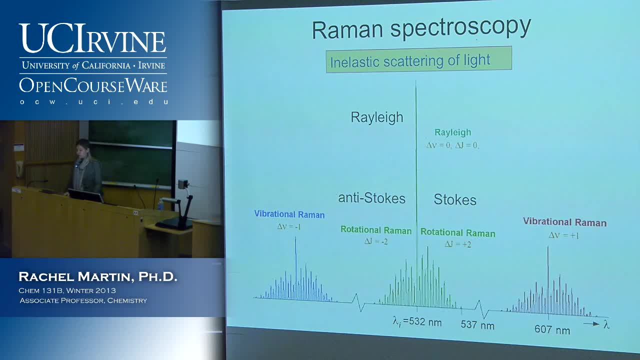 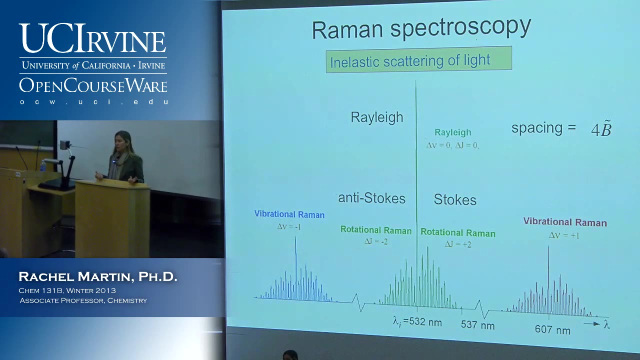 and we need to pay attention. These names are just historical but you'll see them All right. So the spacing between these lines is 4 times B the rotational constant. So remember the spacing between the lines in the direct absorption spectra was 2.. 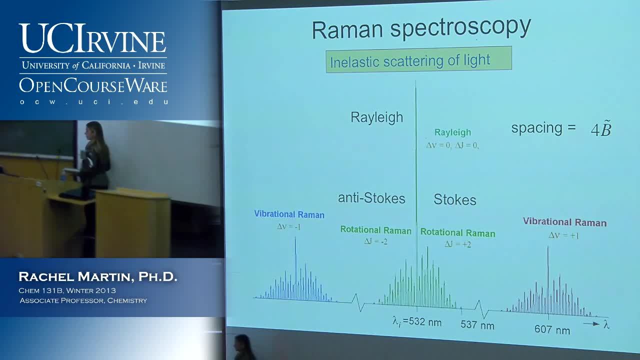 So we're going to have to pay attention to that. So remember, the spacing between the lines in the direct absorption spectra was 2.. So remember, the spacing between the lines in the direct absorption spectra was 2B, And we're going to talk about why that is, hopefully. 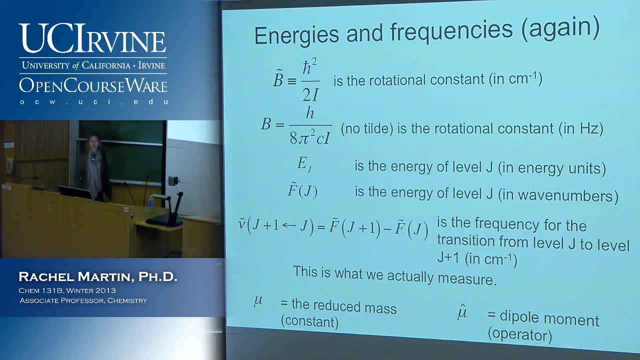 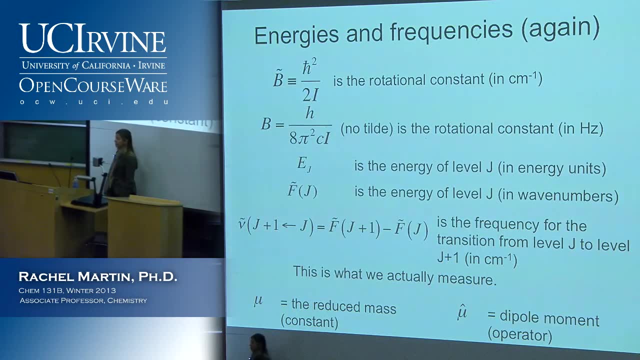 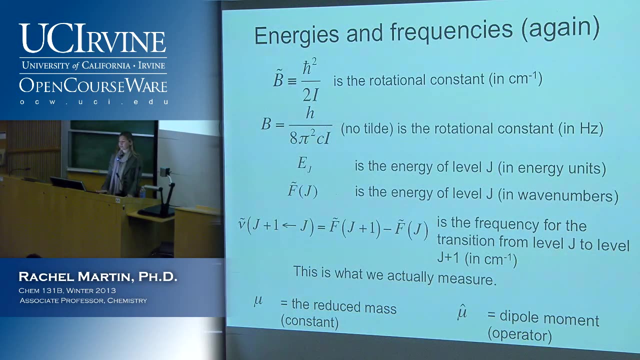 by the end of this lecture. OK, So I want to again put up this description of energies and frequencies. So B is our rotational constant. If it has a tilde over it, then it's in wave numbers And we can also define it in hertz, and somebody asked this question. 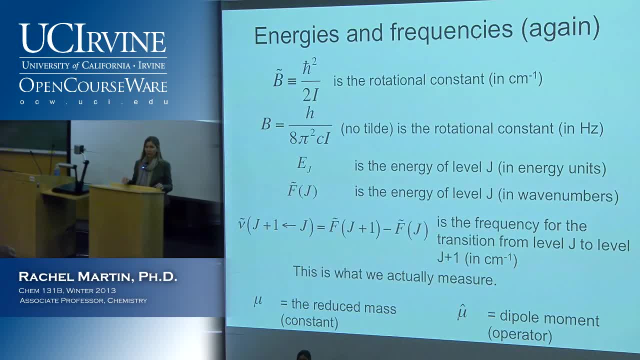 Somebody asked this question, Somebody asked this about this before. I think I had them, you know, inappropriately set equal or something. They're different things. It matters if it has a tilde over it or not, And so you know we can use the fact that E equals HC. 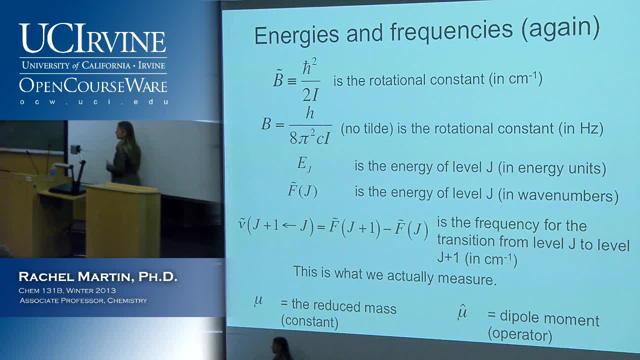 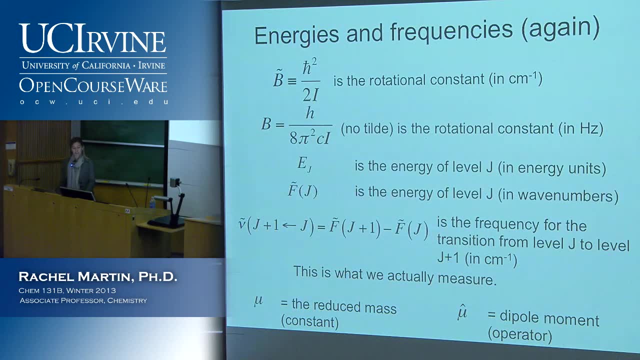 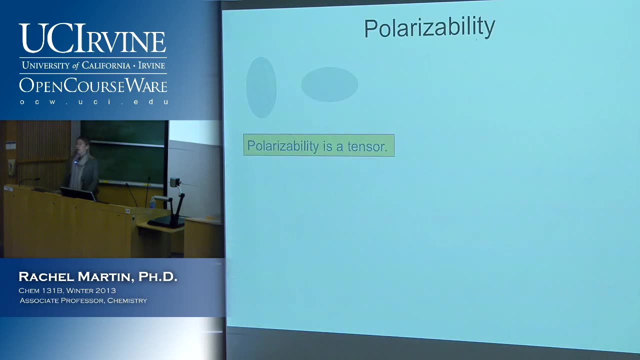 over lambda, to express this in hertz. And then we've also got these energy levels that we talked about before and we don't need to go through again. OK, So we're going to go through this. OK, So how do we know when something is going? 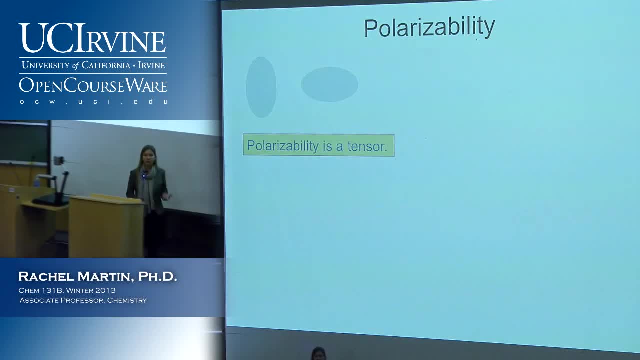 to have a rotational Raman spectrum. So we said that for a direct rotational spectrum the molecule needs to have a dipole moment. So Raman is based on scattering, not absorption. It's a different effect. So it makes sense that we might have different selection rules. 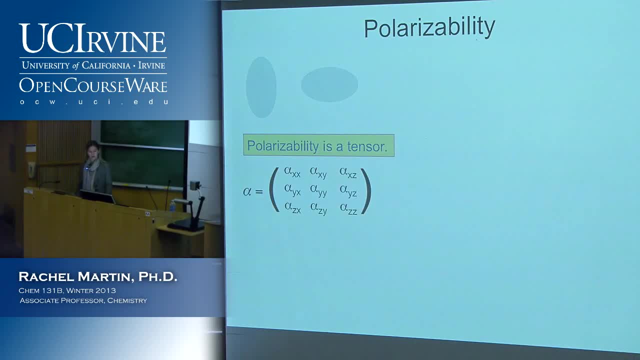 and we do. The gross selection rule for rotational Raman is that we have to have an anisotropic polarizability. So let's talk about what that means. The polarizability is the ability of the electron cloud of a molecule to distort when you put it in an electric field. 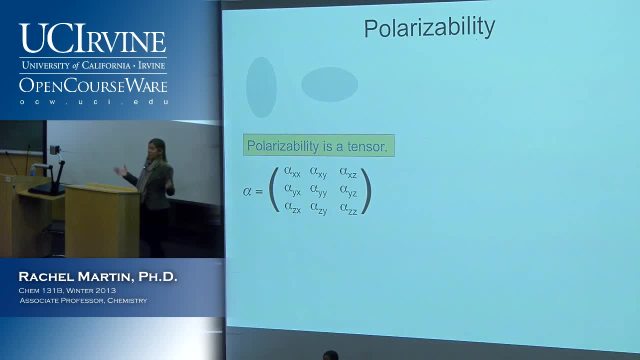 So we're talking about an induced dipole moment. It doesn't have a dipole moment necessarily on its own, but when we put it in an electron field, the electron cloud is, you know, big and can move around a little bit and can get distorted. 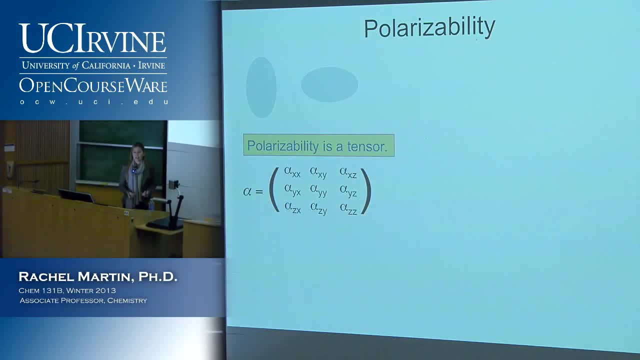 So polarizability is a measure of how much that can happen, And it is a tensor, It's not just a number, So it's represented by a 3 by 3 matrix in 3-dimensional space. Here's a picture kind of illustrating what I mean. 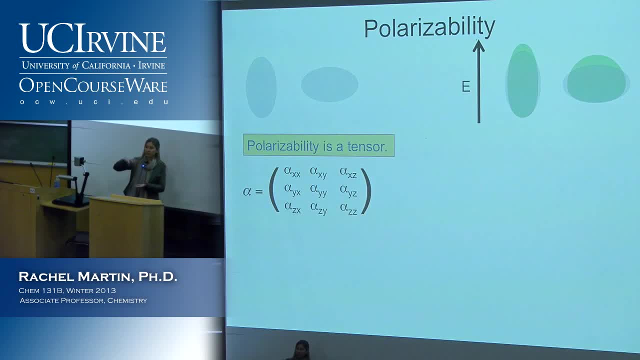 So if we put this molecule in an electric field, that electron cloud is just going to distort a little bit, And some molecules might distort a little, some might distort a lot. That's the magnitude of the polarizability, But we also have to describe it spatially. 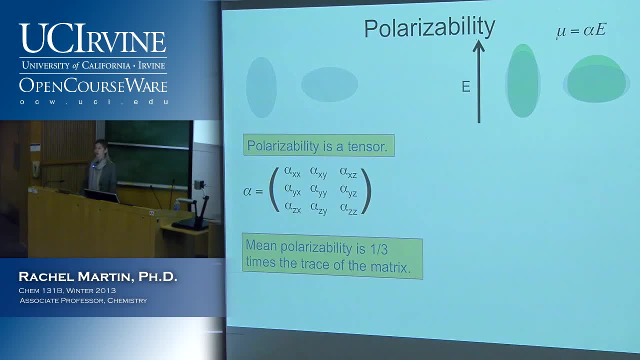 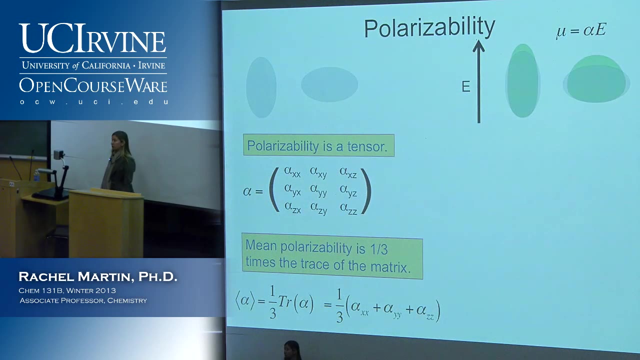 So we can also define the mean polarizability, which is just a number And that is a third times the trace of the matrix. So of course from our group theory discussions you remember how to get the trace of a matrix. 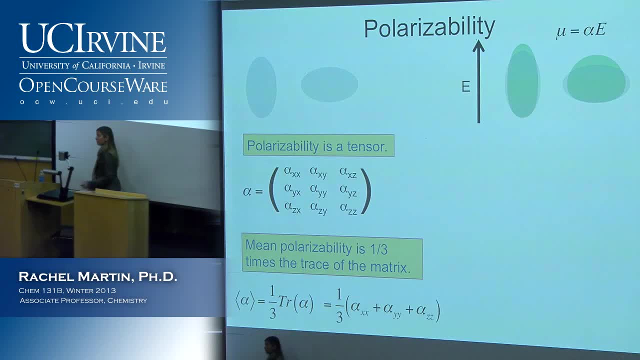 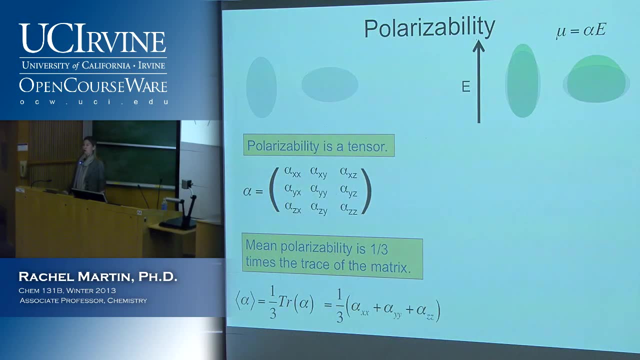 Just add the elements on the diagonal And then if you divide it by 3, you get the mean polarizability, And that's mainly it, And that's mainly useful for comparing, you know, among molecules, If we want to talk about in detail what these things do. 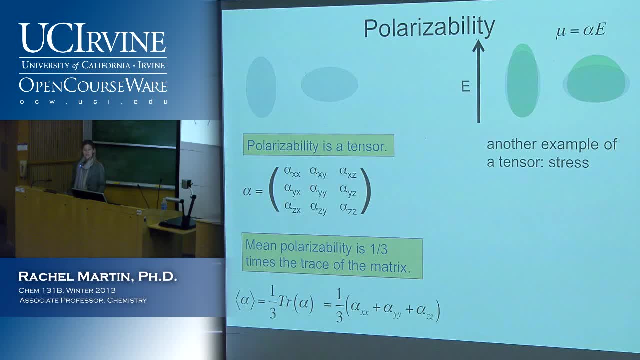 we need to use the full tensor. So just in case it's hard to visualize what the tensor looks like, here's another unrelated example but that at least the engineers have definitely seen before And hopefully it's a little bit easier to visualize. 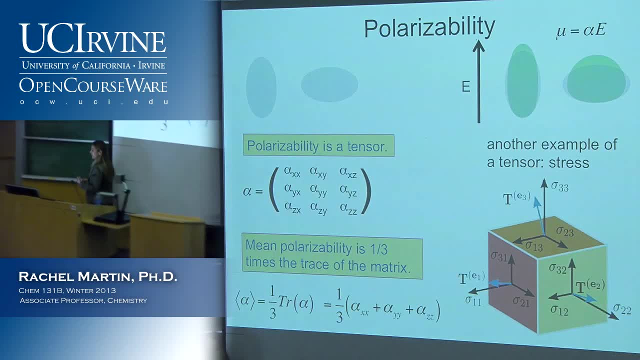 So we're just, you know, we're just looking at the. you know, we're just looking at the. you know, looking at, you know how this property varies in space. So stress is another example of a tensor. 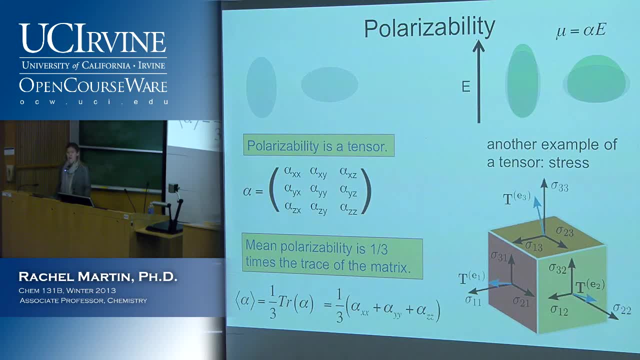 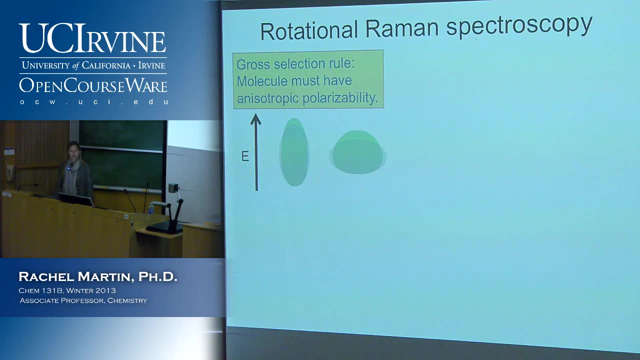 There are lots of them in physics. This is a really important concept and I recommend you know looking up more about it if it's not clear, OK. So we said that our gross selection rule for Raman spectroscopy is that our molecule has 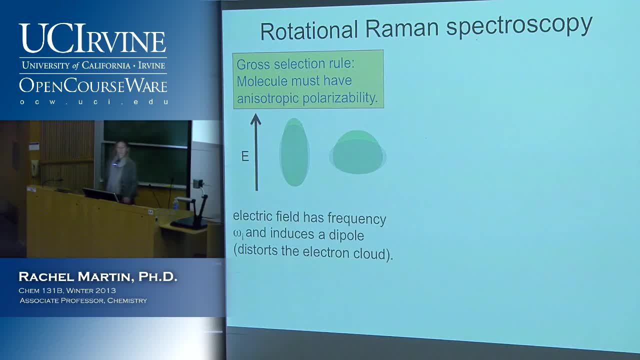 to have anisotropic polarizability. So we stick the molecule in an electric field and it that has some frequency. We can call it omega, so omega I, And it induces a dipole. So here's an expression for our induced dipole. 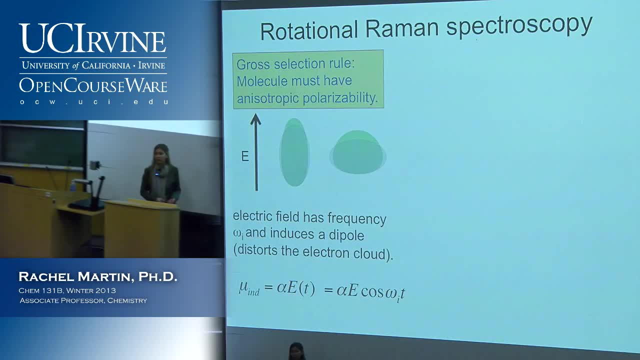 So we have an alpha in front of it which makes sense. That polarizability factor tells us something about the magnitude of the dipole that we can induce with that electric field, And then of course it also depends on the amplitude. 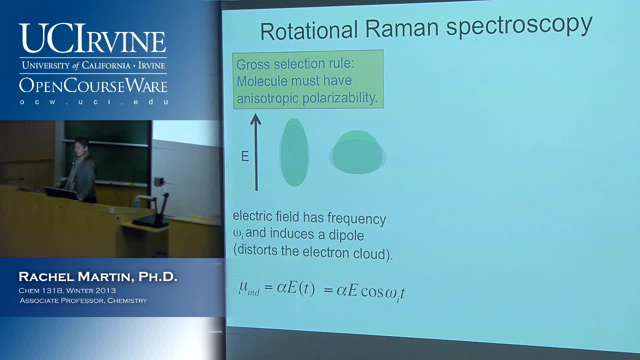 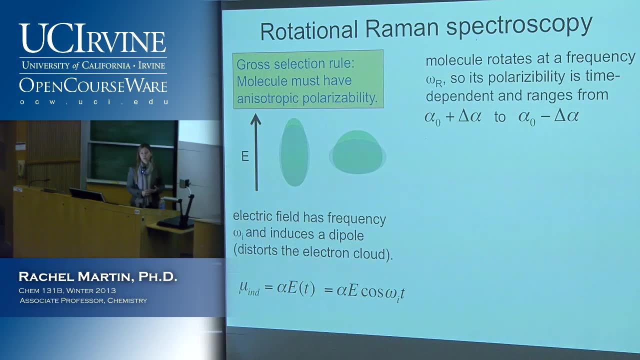 of the field which is varying in time, So it has this time dependence. So omega I is the frequency of the induced field. The molecule is also rotating at some frequency. We're going to call that omega R, And so 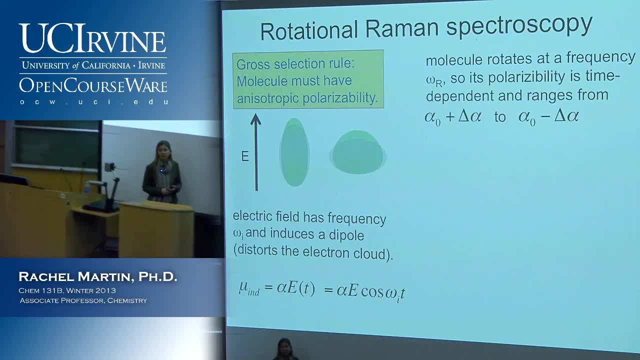 its polarizability is time dependent because, remember, the molecule is anisotropic. So here I drew it shaped kind of like a football. So if the molecule is, you know, has the football standing up with respect to the electric field. 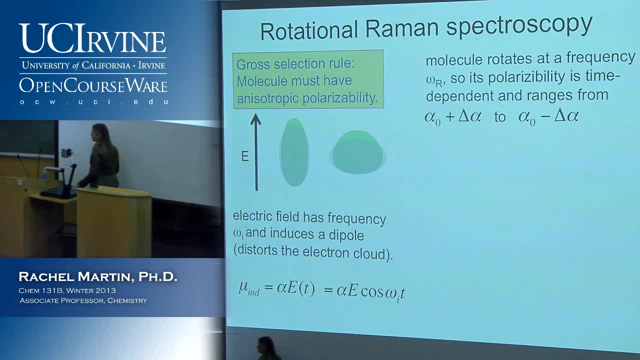 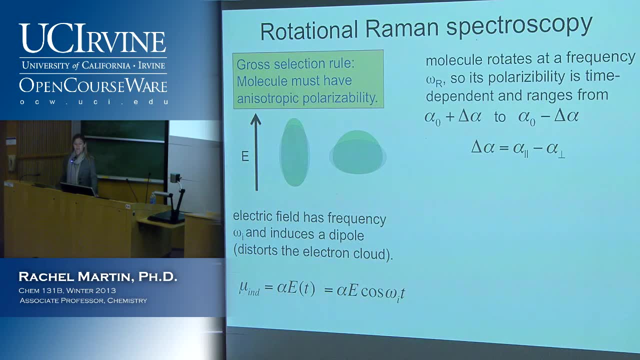 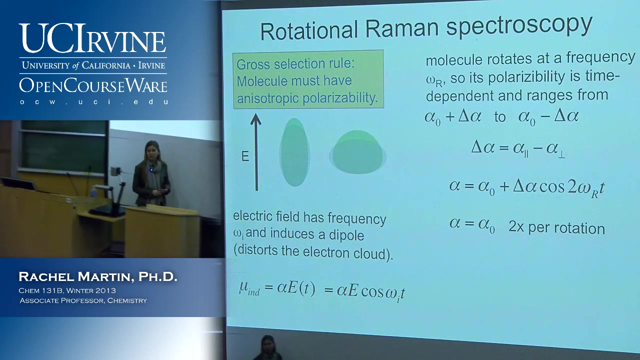 its polarizability is different than if it's lying down, And it ranges from these between these values. So delta alpha is the change in polarizability from the parallel orientation to the perpendicular one, And so we can define its time dependence in terms. 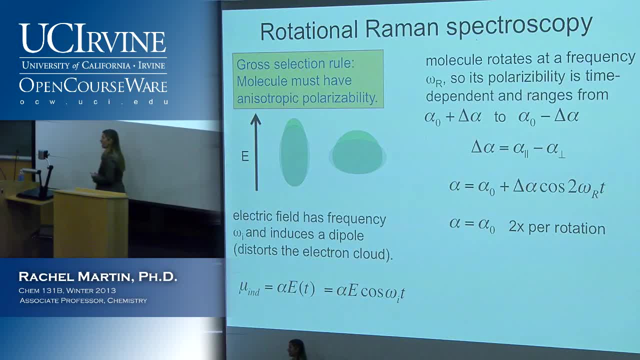 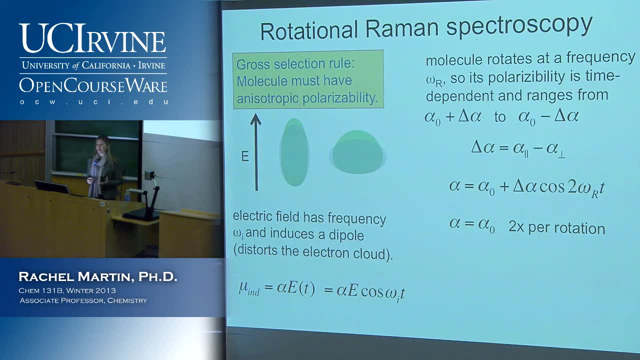 of the rotational frequency of the molecule, And one thing that's important to this is that it comes back to the same value two times per rotation. Why? Because we're assuming that we have small electric fields and it doesn't matter whether I hold the football like this or like that. 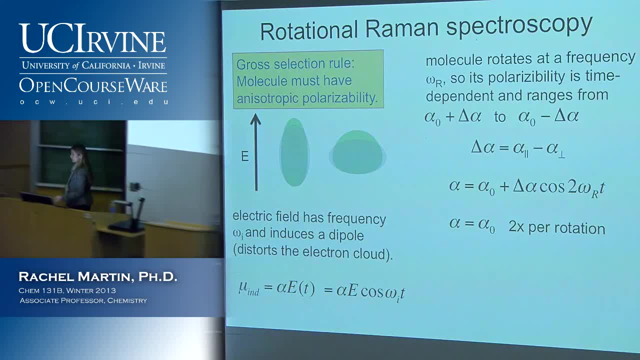 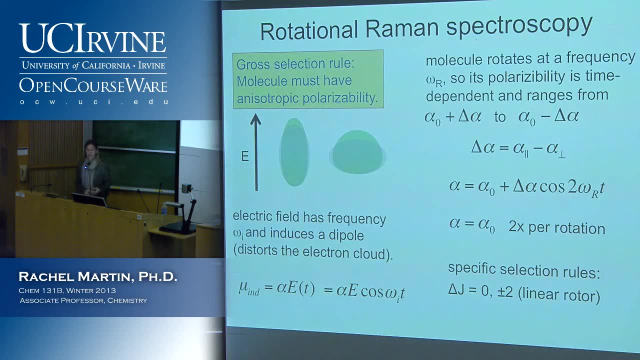 And that's true even if the molecule isn't exactly symmetric, at least for the case of small electric fields, And so the specific selection rule for a linear rotor is that we can have either no change in rotational state or we can have things jumping up and down by two. 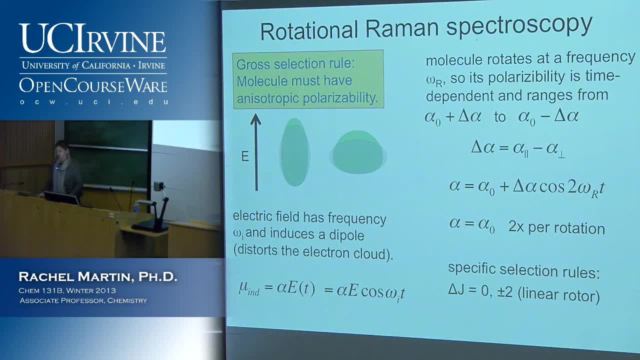 And that's because we get the same effect two times per rotation. So we're assuming that we have small electric fields, So we can have two times per rotation rather than one time. So that's why the specific selection rules are different. 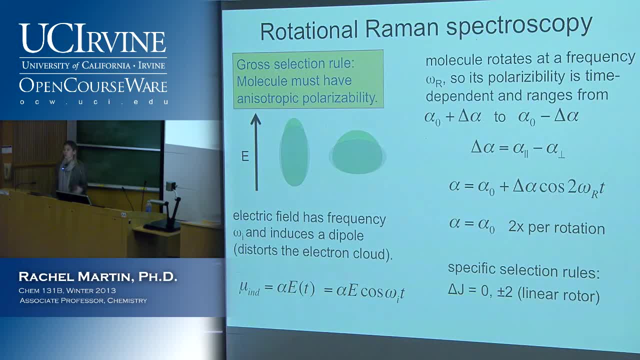 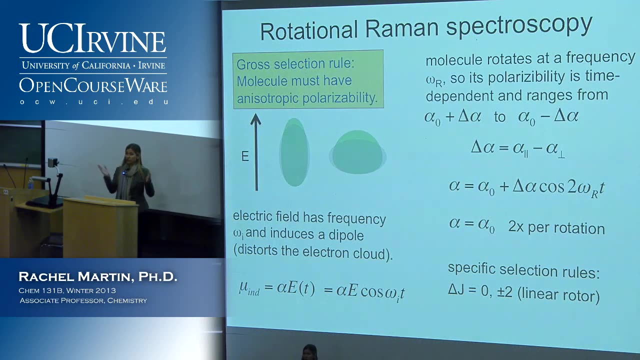 for rotational Raman than they are for rotational spectroscopy. OK, So I also want to point out that if we have this, delta J equals 0, condition that contributes to the Rayleigh line. So what we're saying there is: the photon hit the molecule. 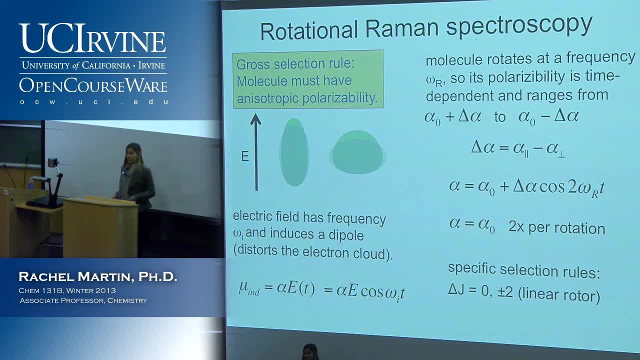 and it just bounced off and it didn't change its rotational state. That's Rayleigh scattering. OK, So we're assuming that we can have two times per rotation rather than one time. So that's why the specific selection rule for small electric. 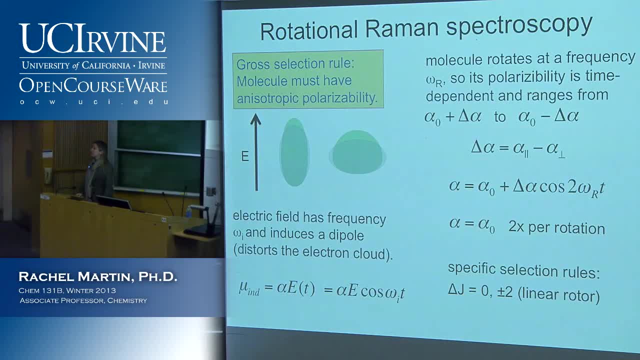 fields is that we can have two times per rotation rather than one time. OK, Yes, Do you have to do this for each individual wavelength of light that you want to measure, So when you actually? so that's a good question. So the question is: do you have to do this for every wavelength? 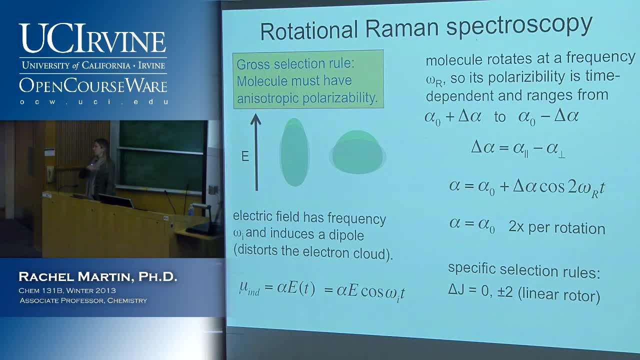 of light that you want to measure. What we would do in a real experiment is just sweep through a whole bunch of wavelengths and see how it responds, which- and we'll see some examples of the spectra later. So essentially yes, but we can learn some things. 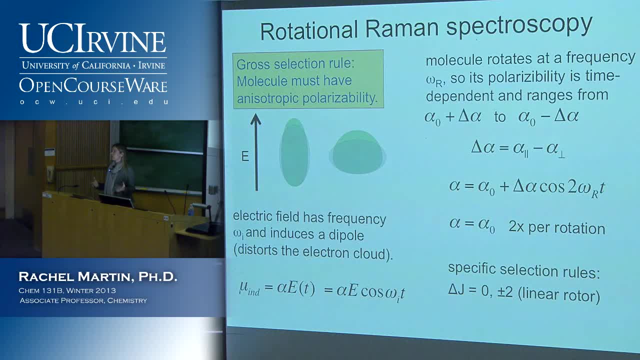 about what the overall spectrum is going to look like without doing that. So if we want to predict what the spectrum looks like in a qualitative sense, we don't need to do it at every wavelength. If we want to know specifically what it looks like, then we do. 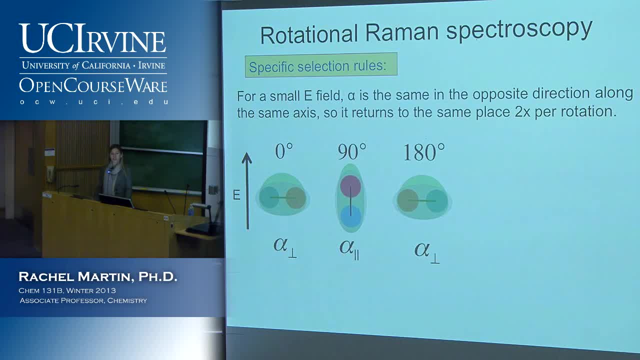 OK, So here's just a picture illustrating what I just said, just in case. So we have our electric field, We start out with this thing in the perpendicular orientation and then, if we rotate it 90 degrees, we're going to have a little bit of a problem. 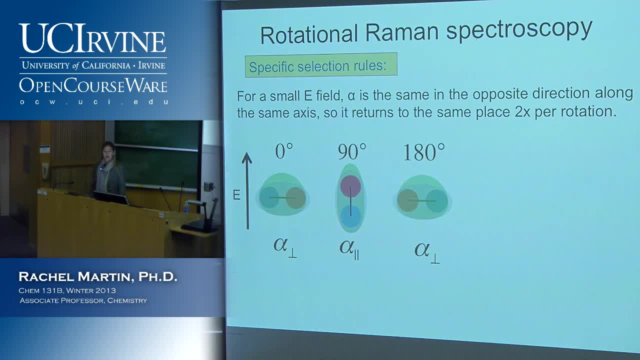 If we rotate it 90 degrees, now it's parallel and the polarizability is different, And then, as it keeps going around, you know now the blue atom and the red one are flipped, they might be different. I'm saying I don't care about that. 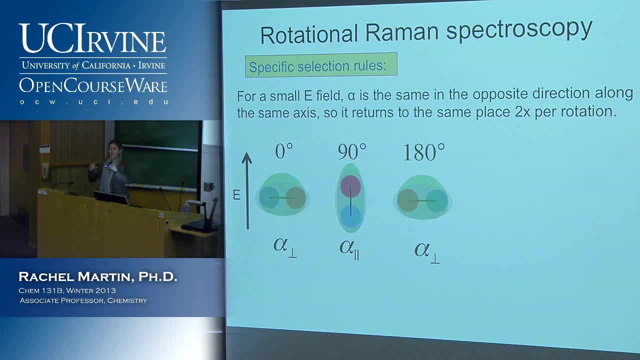 It's a good approximation that we're just looking at the polarizability this way versus this way, And so that's why we get the same thing two times per rotation and that leads to that selection rule, And we're not going to talk about this. 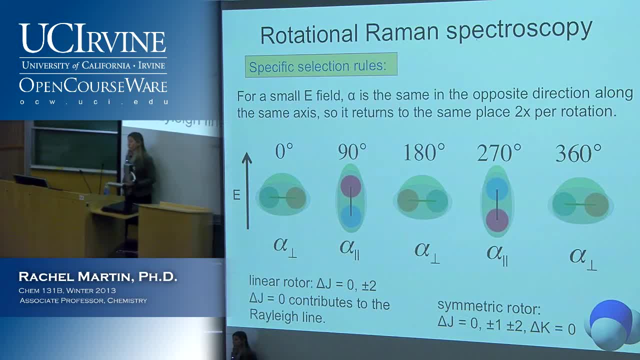 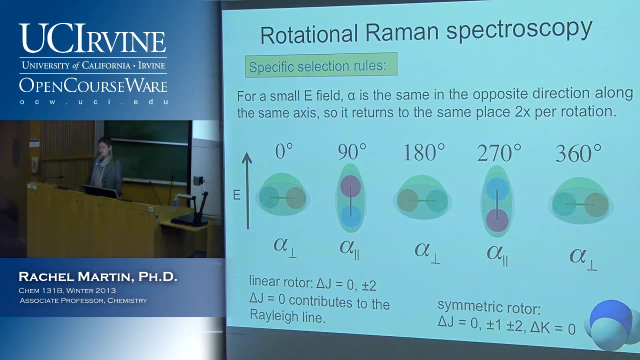 This right this minute, but I'm just throwing it in here for future reference. For a symmetric rotor, we have the same conditions for delta J and delta K equals zero. OK, So I am going to yes For this. is this like the same? 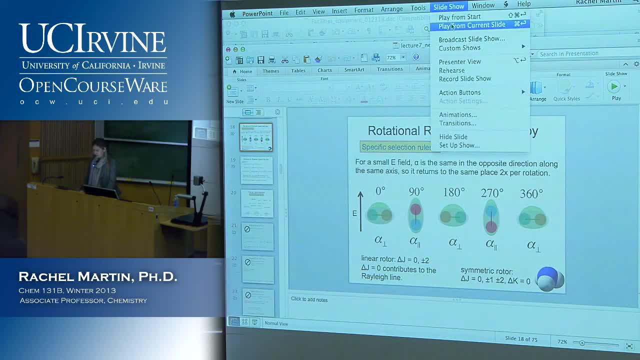 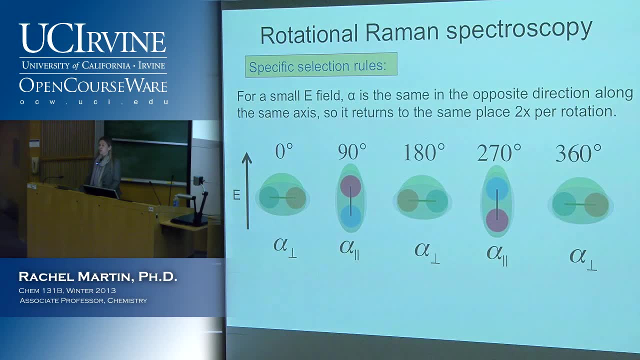 Yes, It's like all the electrons are basically being pulled in one, like in opposite directions. or is it just the bond that's actually stretching, or is it The bond isn't really stretching? That would be vibrational spectroscopy. It's just that the polarizability is changing. 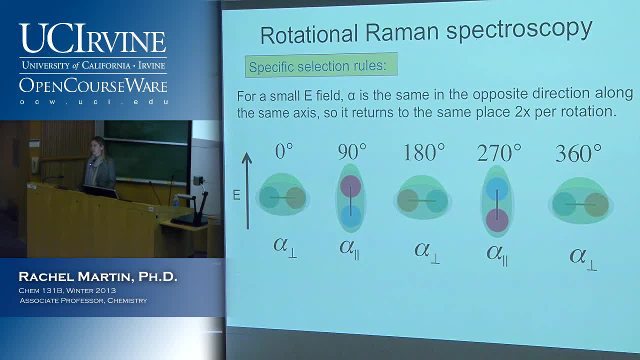 a little bit. It's just like the electron cloud is deforming. OK, So the entire electron is kind of shifting. Yeah, It's just kind of moving around, It's making an induced dipole, but it's not changing the bond length. 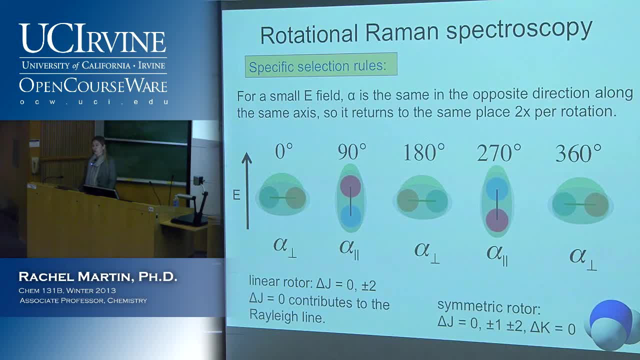 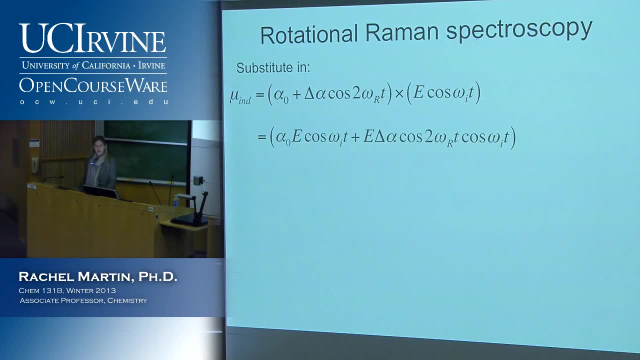 Oh, That would be vibrational and we'll see that. We'll see that later on, OK, So if we substitute in what are, if we substitute in these expressions into our expression for the induced dipole, what we get is: 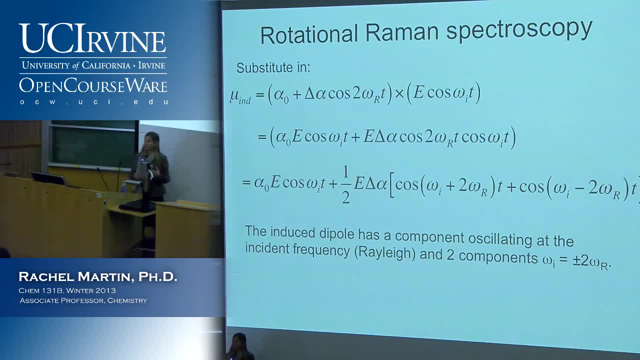 that it has a component oscillating at the incident frequency. So that's the electric field that we're putting in and that's why we care about that frequency. That's the Rayleigh line, And then we also have the you know, the you know. 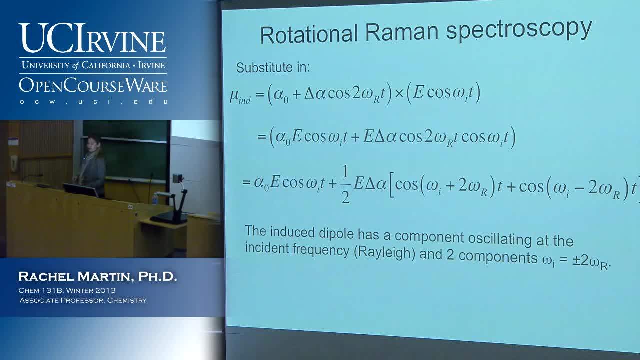 we also see two components that have to do with, you know, that- incident frequency plus or minus 2 times the rotation frequency. So that's how we get that pattern where we have the Rayleigh line in the middle and then all of those little spikes. 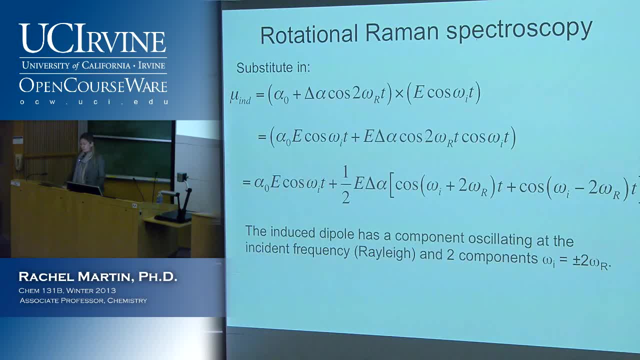 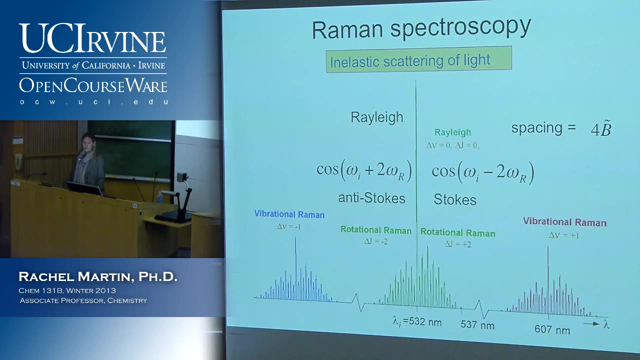 for the individual rotational transitions on either side of it, And those only occur if delta, alpha, or the difference between polarizability when the molecule is parallel versus perpendicular, doesn't equal zero. And so here's that picture again, showing where these frequencies fall out. 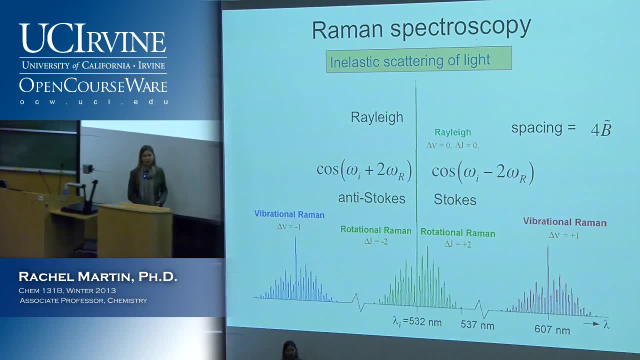 So that's how we know where they are, We know what they look like, We know why the selection rules are the way they are. We're going to talk about these selection rules and how this relates to symmetry in more detail later, after we go. 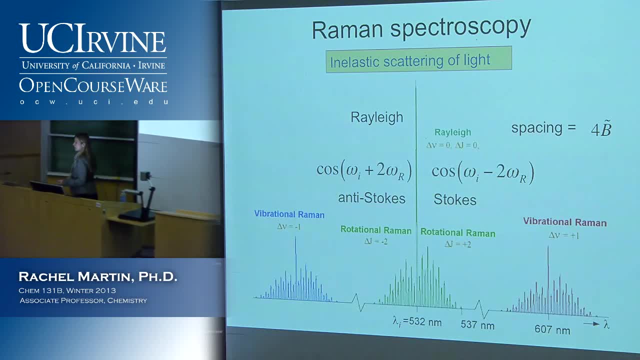 through vibrational spectroscopy. But I think for now we're going to talk about you know, I think for now we are going to move on to vibrational spectroscopy and talk about the basics of that. Does anybody have any questions about rotational Raman? 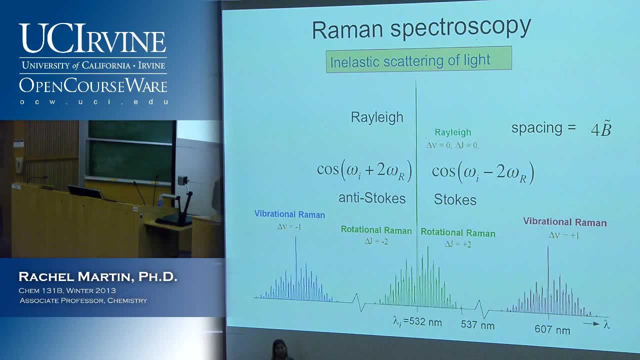 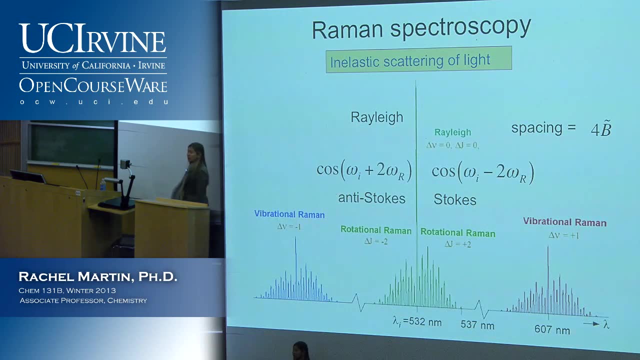 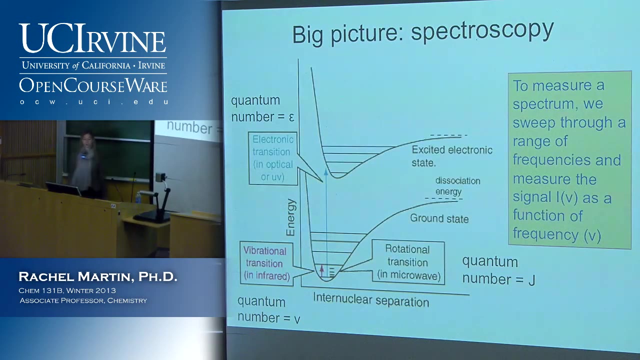 and the difference between that and absorption, rotational spectroscopy. OK, Let's talk about the next level up in this diagram. OK, So so far we've been looking at these, these two diagrams. OK, So so far we've been looking at these. 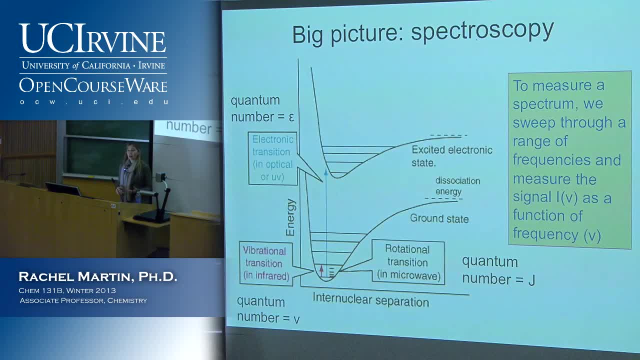 these tiny little rotational transitions that don't take very much energy and that are, you know, honestly, not all that useful for telling us about properties of the molecule that we care about as chemists. Let's move on to saying: OK, now we have more energy to put in. 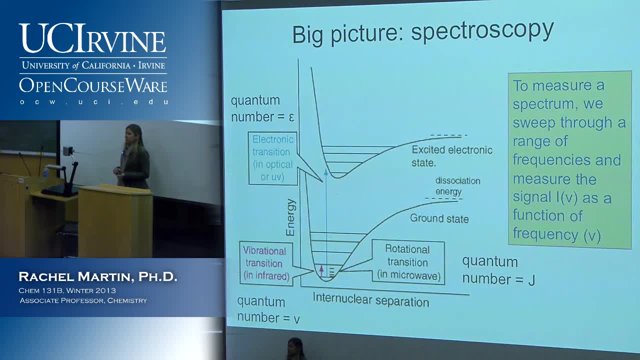 We're looking at infrared and we can excite vibrational transitions. This type of spectroscopy is fantastically useful, and people use it all the time in chemistry too, To characterize all kinds of things, and we'll talk about some specific applications. So now we're in the IR region of the spectrum. 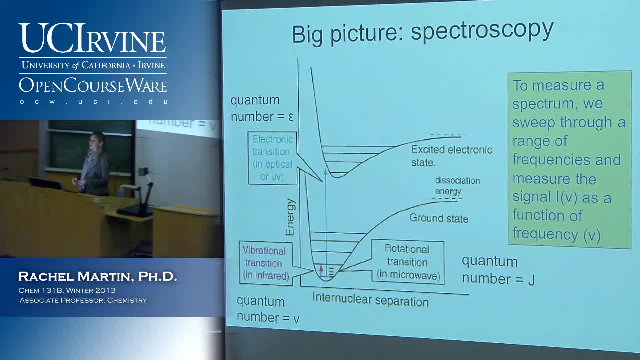 We're exciting vibrational transitions and I should mention that you know we will talk about absorption spectroscopy and Raman. When people just say Raman spectroscopy and they don't specify what kind it is, they're talking about vibrational Raman. 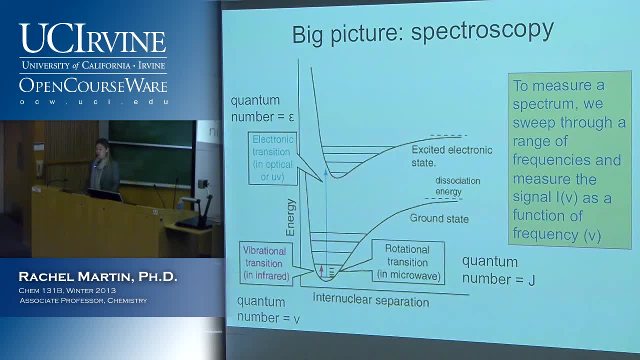 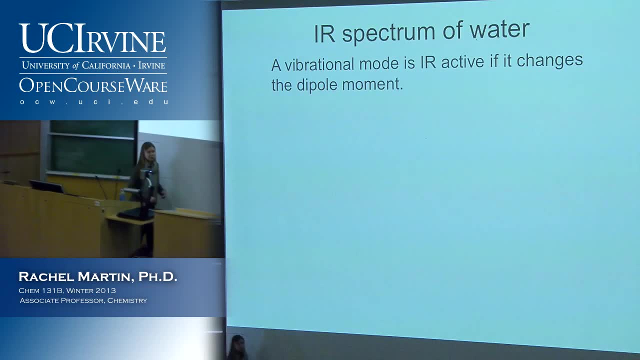 As we just saw, rotational Raman exists too, but vibrational Raman is much more commonly used. OK, So let's talk about the selection rules first, because I think it's pretty intuitive, and then we're going to move on to going through a lot of the details. 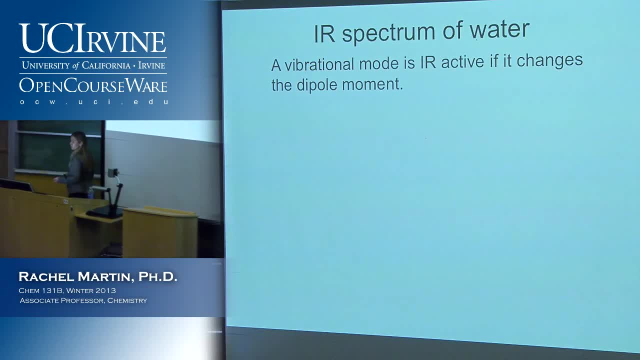 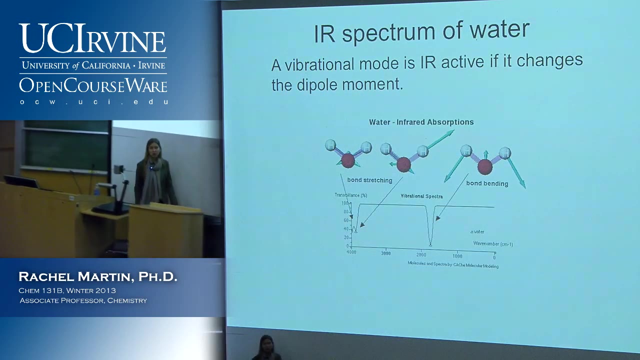 about what you actually do with this. So a vibrational mode of a molecule is IR active. That means we can see it. It's actually changing the dipole moment of the molecule. So water obviously has a dipole moment. but what's important, 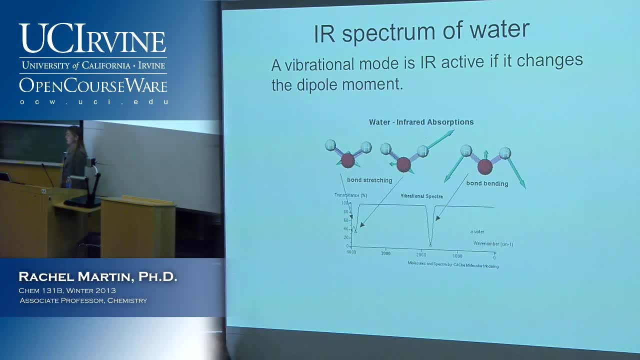 for the molecule is that it's actually active. So what's important for being able to see these modes is whether the motion of the molecule actually changes the dipole moment. So if we have a water molecule, you know we have the oxygen. 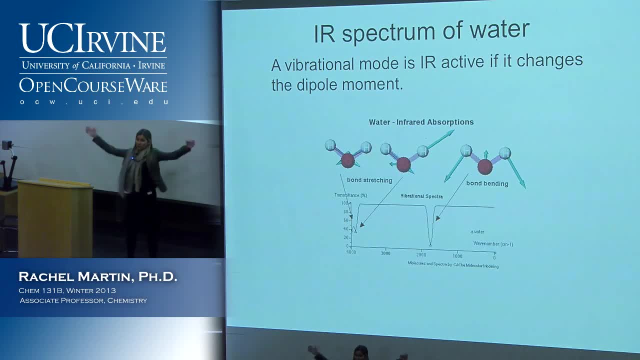 and the two hydrogens. those bonds can stretch and they can do that in a symmetric way, like they can move together in phase with each other, and that obviously changes the dipole moment. right, Like those bonds are getting longer, things are spreading out. 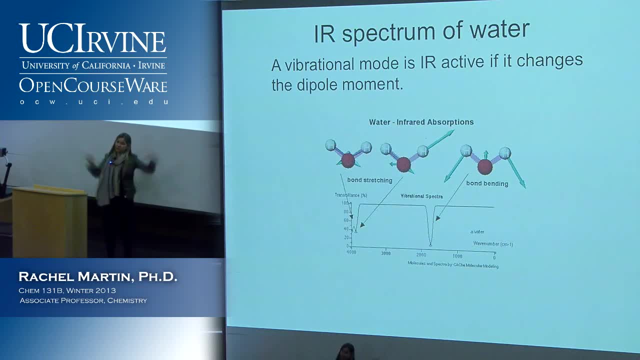 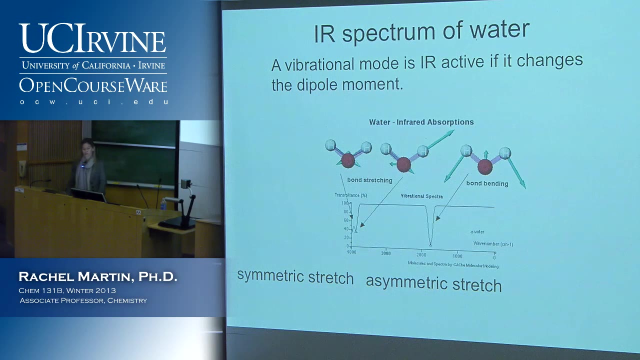 They can also do it in an asymmetric way, so like this: and that changes the dipole moment too, and you can also have them bending, And so we can see pretty intuitively that all of these motions are going to be IR active and change the dipole. 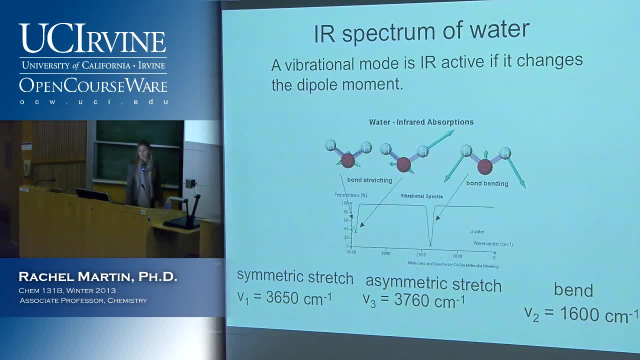 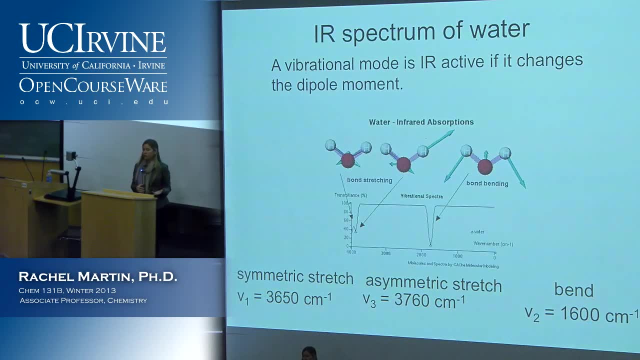 Incidentally, here's where they show up in wave numbers. What we're going to learn how to do is use our group theory operations to figure out which of these motions are active. So we're going to use the wave numbers Which vibrational modes are infrared and Raman active. 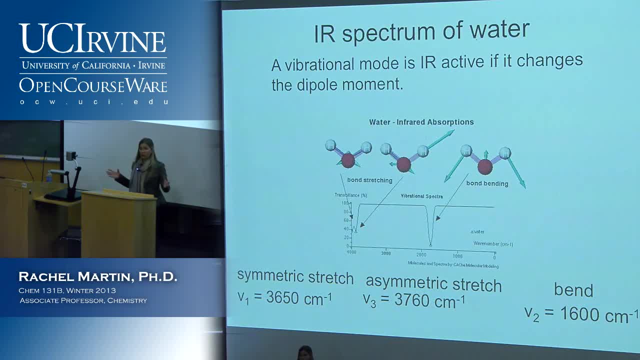 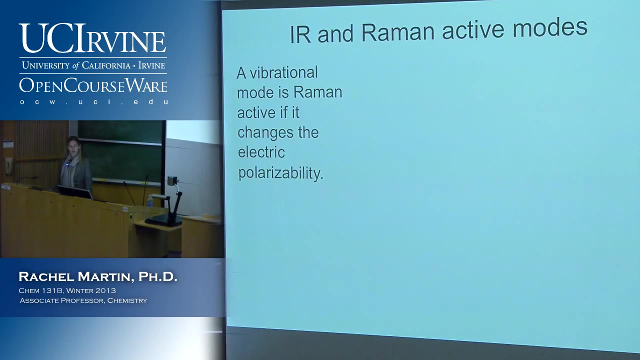 Because in the case of water, you can do the little vibrating water molecule dance and figure out which ones are going to change the dipole moment. It's not always very obvious, particularly if the molecule is at all complex. So how do we know if something produces a vibrational Raman? 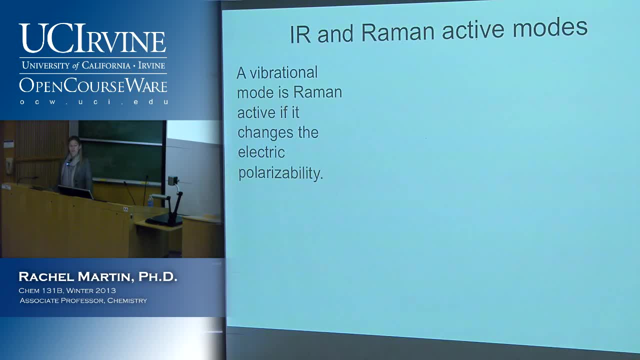 spectrum There. the vibrational mode is going to be Raman active if it changes the electric polarizability, and we just learned what that is. So CO2 doesn't have a dipole moment, but if we think about its polarizability, the size of its electron cloud, 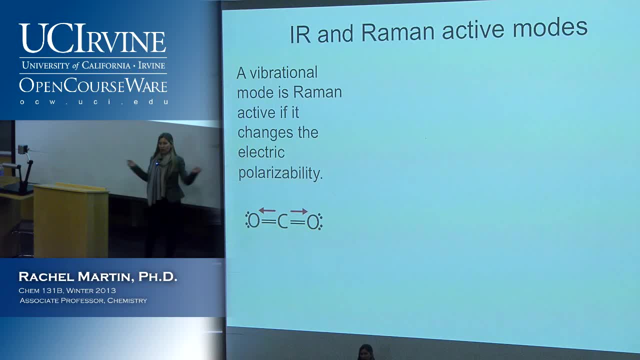 if we have the mode where the two oxygens are stretching, that's going to lengthen the overall molecule. So now we are getting to the case where the bond length is changing right, Because we're talking about vibrations. The overall molecule is lengthened. 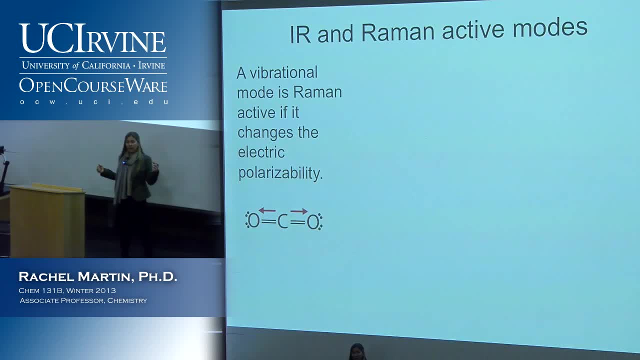 lengthening and shortening as it vibrates and that is going to change the shape of the electron cloud. So the polarizability changes and the molecule is Raman active. So we're going to see that mode. You can also imagine modes that aren't really going. 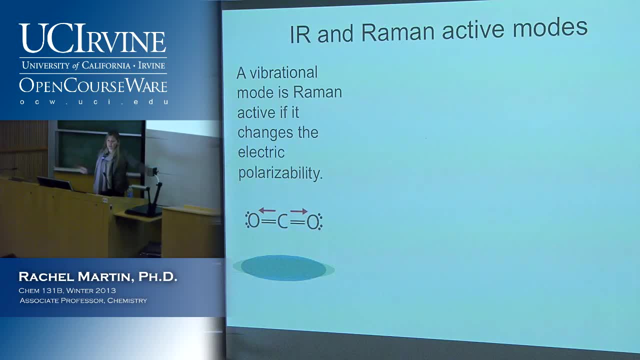 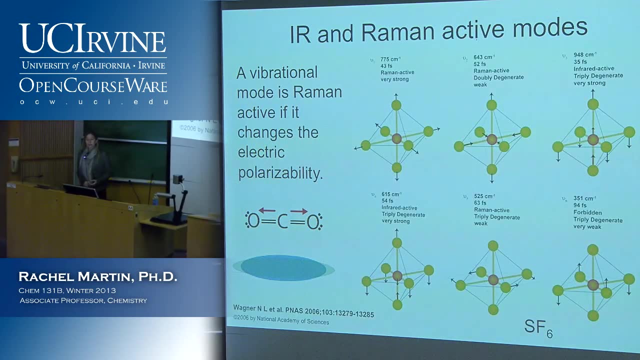 to change the polarizability. So, for example, if this thing goes in an asymmetric fashion, that's going to look the same right, So not active. So now let's. we're not going to analyze these in any great detail, but let's just look. 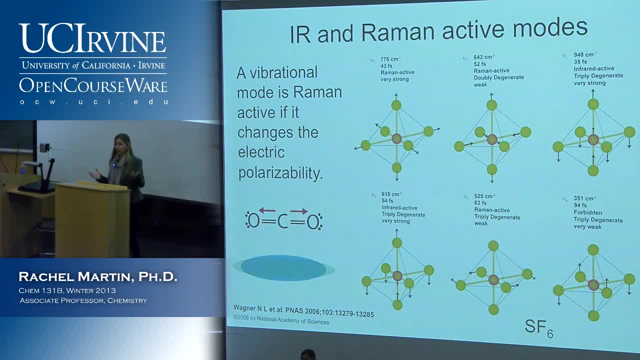 at the vibrational modes of SF6.. So here are a bunch of them, and my objective here is to convince you that for molecules that are simpler than something like water and CO2, you don't actually want to try to visualize all the possible vibrational modes. 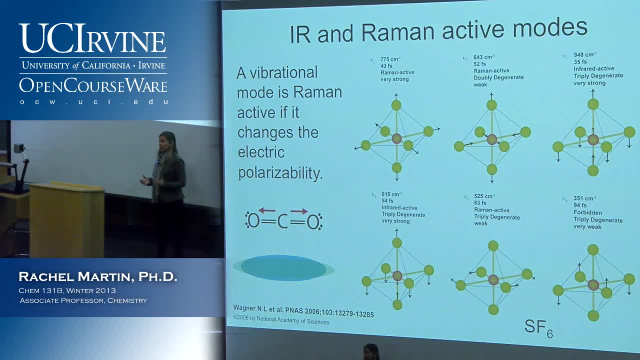 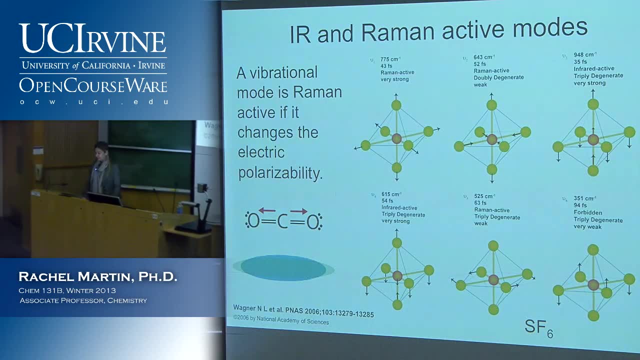 and decide whether they change the dipole moment and or the polarizability. So we need a better way to do this and we're going to use group theory. So remember I said when we talked about bonding and we're doing, you know, something that looks. 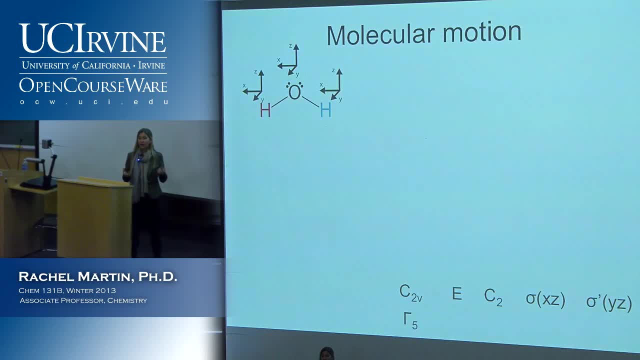 like the hardest thing in the world to get answers that we already know. That was like martial arts practice. So you want to be able to do this over and over again in a situation where it doesn't matter, so that when you get to the problems where it's not obvious. 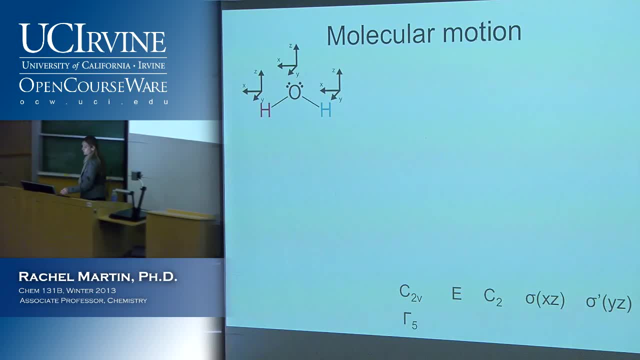 you can do it automatically. So here's what we're actually going to do. So we're going to do this. We're actually going to use this for where we need the answer, All right, So when we're talking about molecular motion and we want, 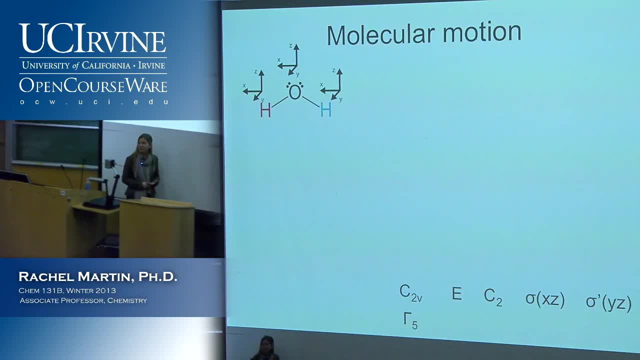 to use group theory to describe it. our basis is now a little x, y and z coordinate system on each atom. Why So? when we're talking about bonding, we set up our basis so that the objects we were looking at had the symmetry of the bonds. 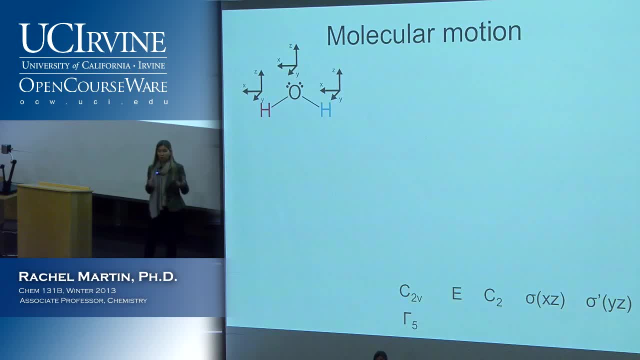 Well, now what we care about is how those atoms in the molecule are moving, Are moving relative to each other, And so we're interested in looking at the, you know, the spatial coordinates of each atom. So that's how we set up this basis. 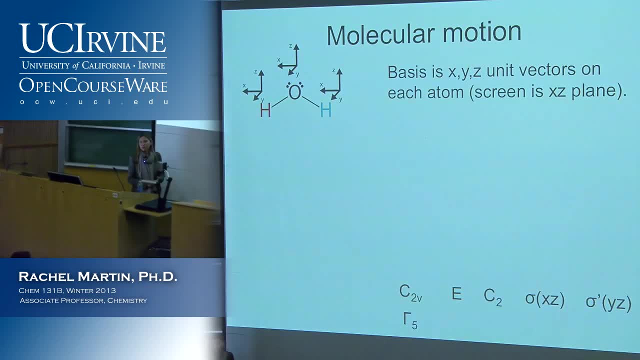 So we have our little x, y and z unit vectors on each atom, And so you can see what's coming. If I set up the transformation matrices for all of these things, I'm going to get huge matrices because we have nine elements. 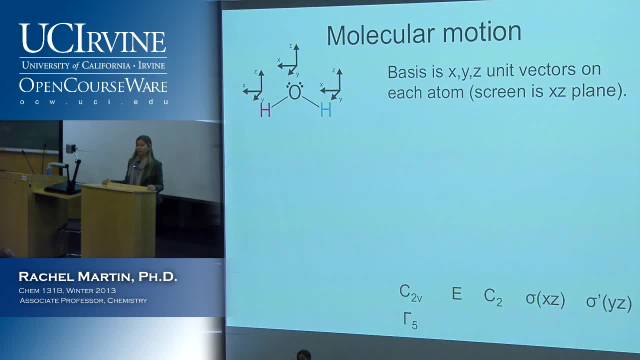 in our basis for water, So I'm not actually going to do that. You can do it if you want. It works fine, But what I'm going to do instead is use the shortcut where we look at what changes and what doesn't change. 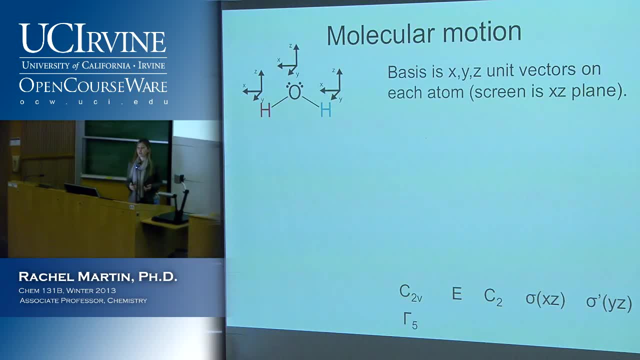 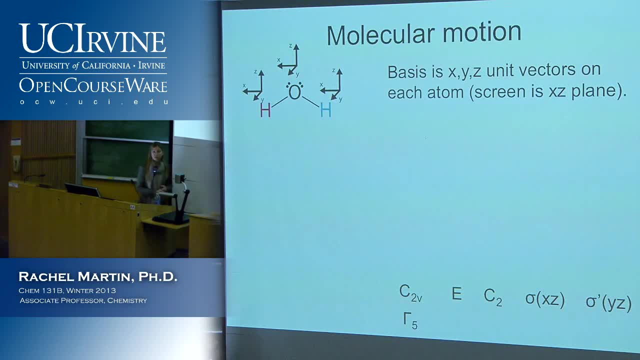 if we have something that doesn't change, it contributes plus 1 to the character of the operation. If it changes sign, it contributes minus 1.. And if it switches places with another element in the basis, we get zero. So that's what we're going to do. 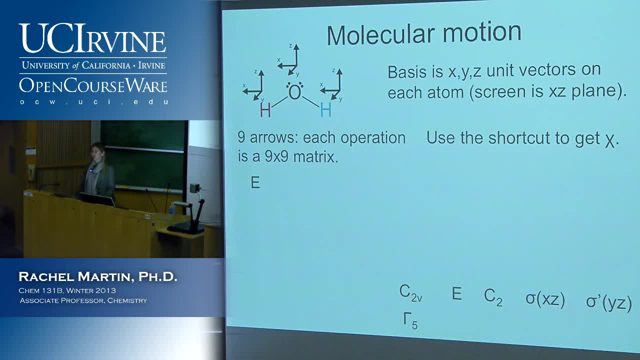 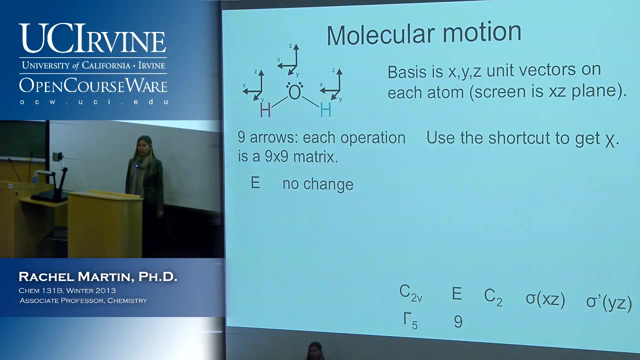 And again, you can write down the 9 by 9 matrices if you want to, but enjoy that, OK. So down here on the bottom we have our representation for C2V, the point group of water, and we're going to look. 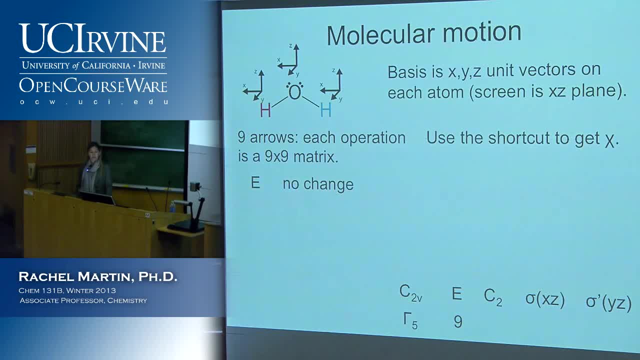 at what character we get under all of these operations. So if we do the identity, obviously nothing changes. So we get 9 for the character. So that's what we're going to do. OK, Now let's do a C2 rotation. 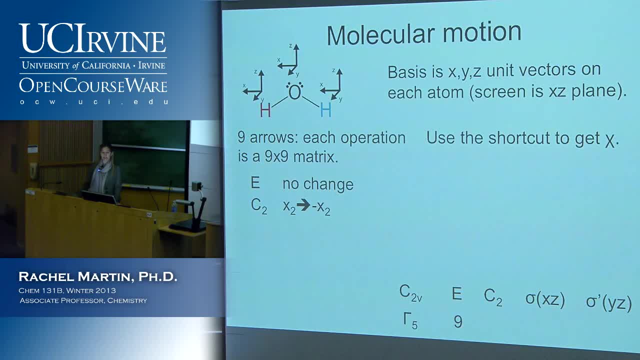 So remember the way I defined this: the screen is the XZ plane, So X and Y are changing sign, Z stays the same. So what do I mean by X2,, Y2, and Z2?? Those are for the oxygen atom. 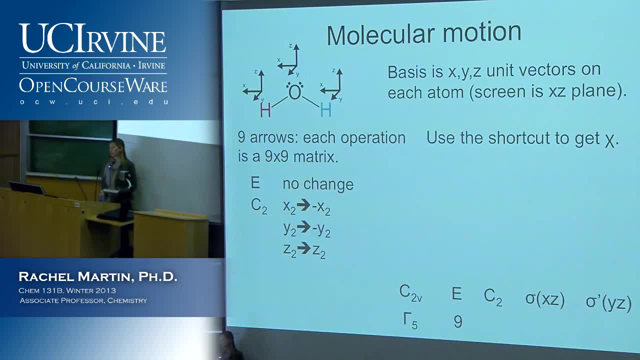 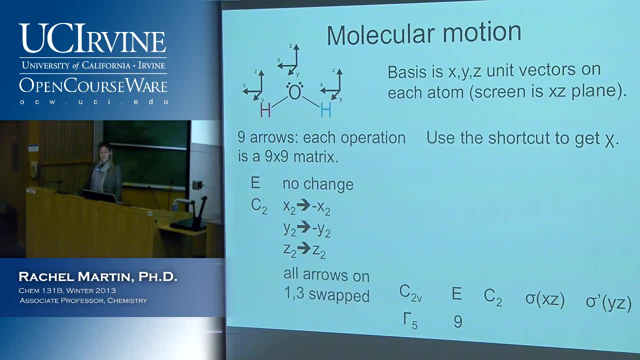 So the red hydrogen is 1,, the oxygen is 2, and the blue hydrogen is 3.. So the little unit vectors in the middle change sign And all the arrows on 1 and 3, the hydrogen atoms get swapped. 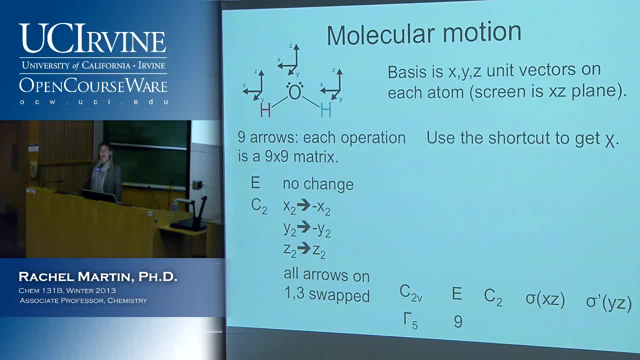 So they contribute zero, And so I'm going to add up all of those little vectors. So we get two of them contributing minus 1 because they change sign, One of them contributing 1 because it stays the same, And then a bunch of zeros. 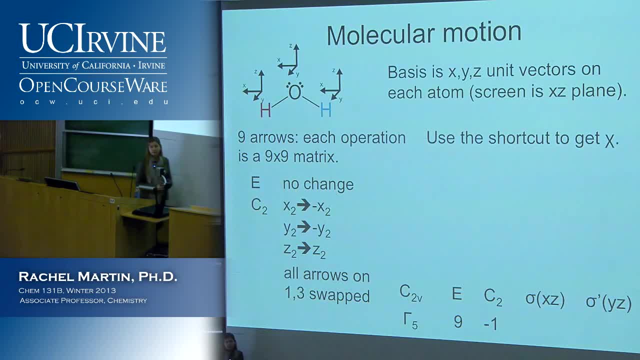 And that all adds up to minus 1.. What do you think? Anybody have any questions about that? Yes, Can you explain how they are all zeros for the agents? Sure, Because, remember, we said that if something switches into another element of the set, it contributes zero. 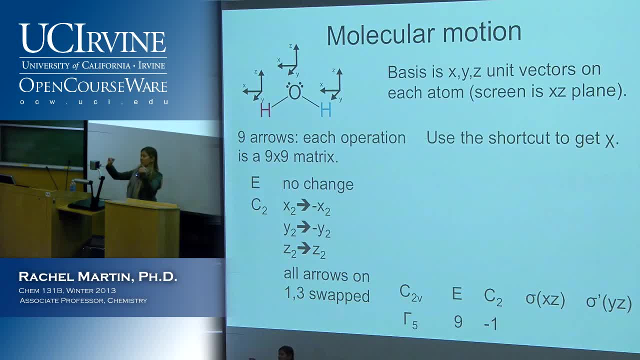 So when I do a C2 rotation, my oxygen is in the middle and the hydrogens are on the sides. They swap around. So the oxygen that was here is- or sorry, the hydrogen that was here is now over there. 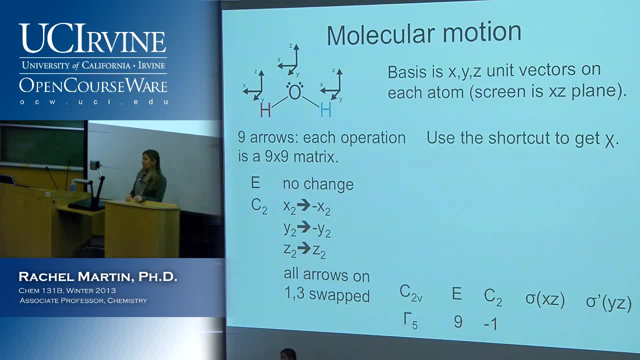 And so Orientation for like the X is like going to be on that direction, or is the orientation for the axis not matter? Well, but it's not. Remember we have a different axis system defined on each atom, because that's our basis. 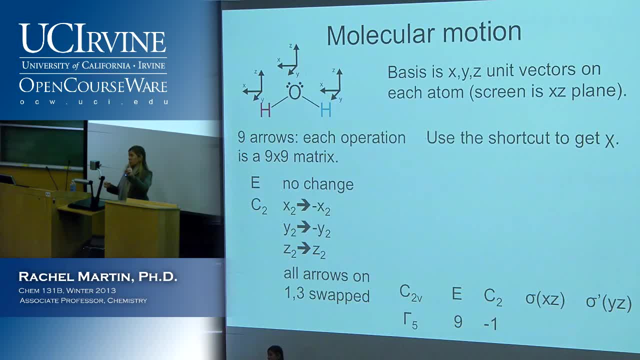 So the X that's over here was the X for hydrogen 1, and the X that was over here is the X for hydrogen 2, and they change places So they get zero, Whereas the one in the middle it just flipped around and so it changed sign. 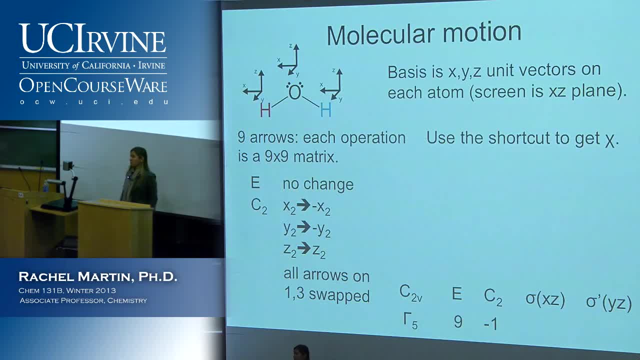 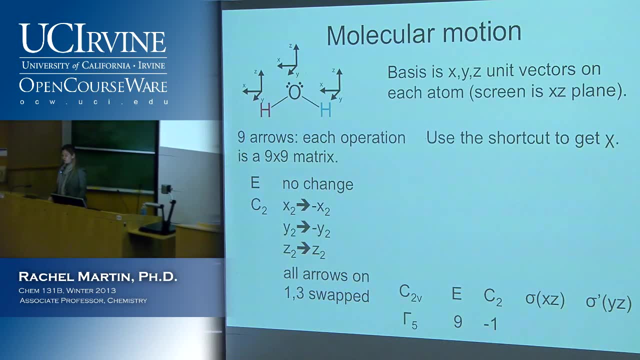 It stayed in the same place and changed sign, as opposed to swapping places. So we are going to spend some time on this. We're going to go over it in more detail next time. I think I'm going to stop here, just because I want. 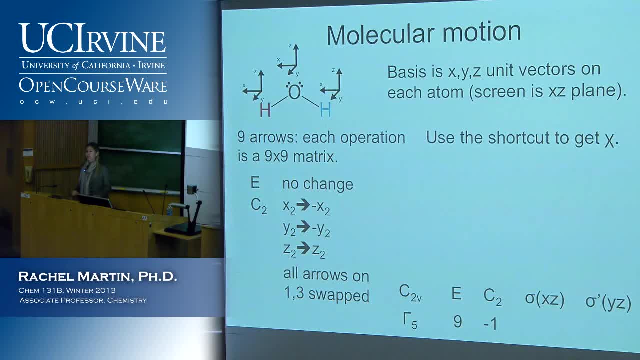 to give you a little bit of time to think about this, But we still have four minutes and I have some other stuff I need to say, So you don't have to run away immediately. I want to point out that I have posted a bunch of practice problems. 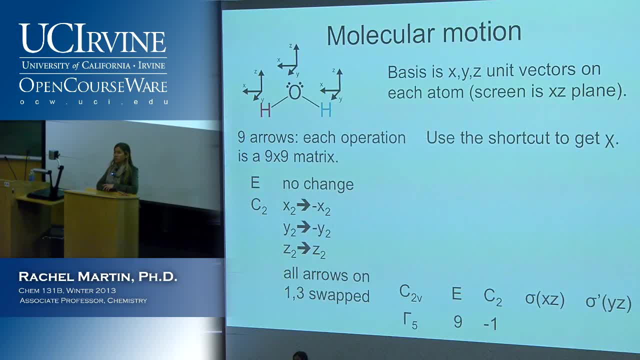 So I posted some problems having to do with direct notation because some people asked for some extra practice with that. There's also a tutorial that I found you know, sort of explaining a little bit more about how to deal with direct notation. I am going to have Thursday office hours. 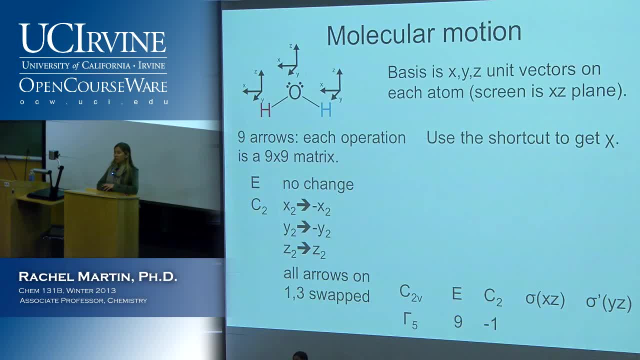 They're going to be 2.30 to 3.30.. So it's not possible to make everybody happy as far as the timing, But I'm at least trying to sandwich it between two classes, So maybe you can just come for the first half or the last half.